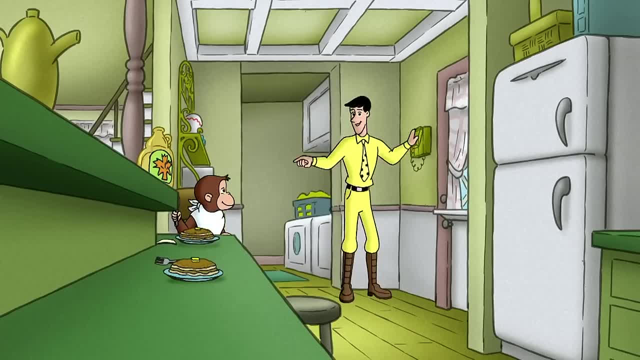 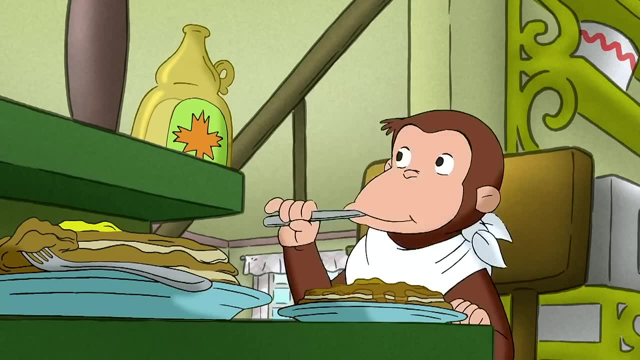 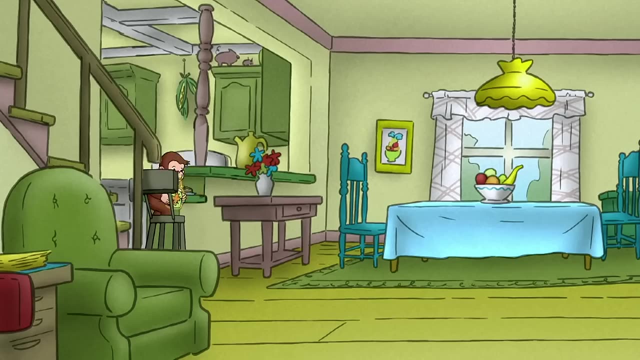 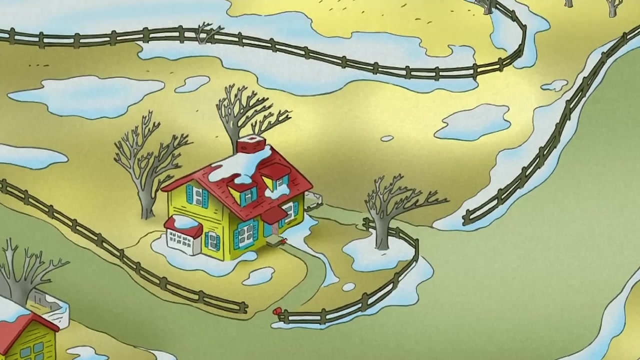 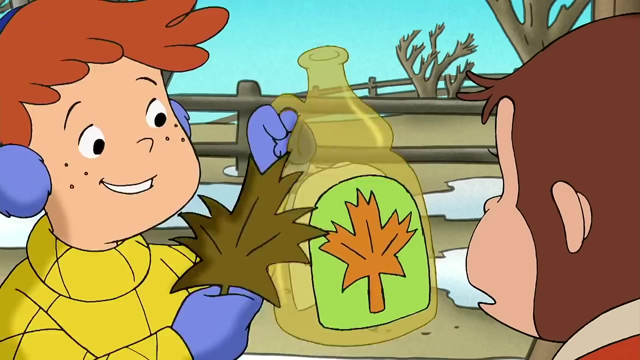 I'll get it. Eat them while they're hot and soggy. Oh Wait, They weren't out of syrup, They had plenty of trees. All he had to do was tap them. But some trees were just right And he didn't like them. 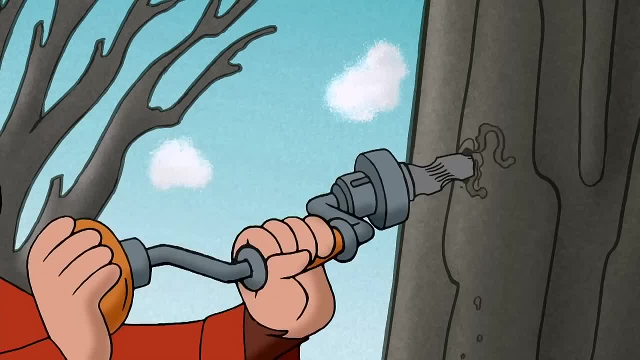 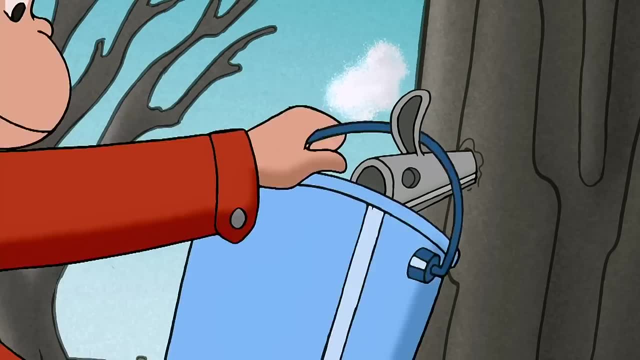 So he started to get upset. Well, he's doing better now. He's called George the Old Teenage Mouser, And George wants to put a party. George doesn't want to do it, So he'd better be a good boy. 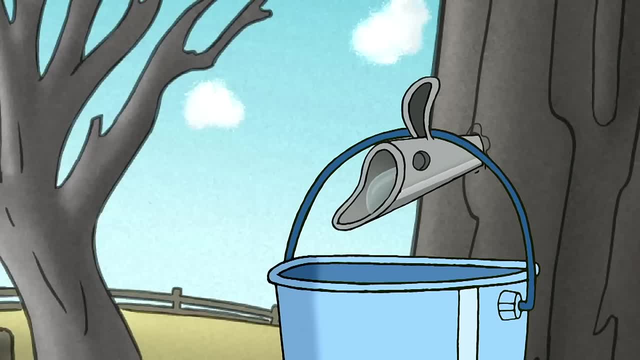 He thinks getting that streak's funny. Yes, yes, But being a little lonely's not helping Soon. you'll learn how to be a good boy, And when you become a good boy you'll be a good person, And then you'll be able to do your job better. 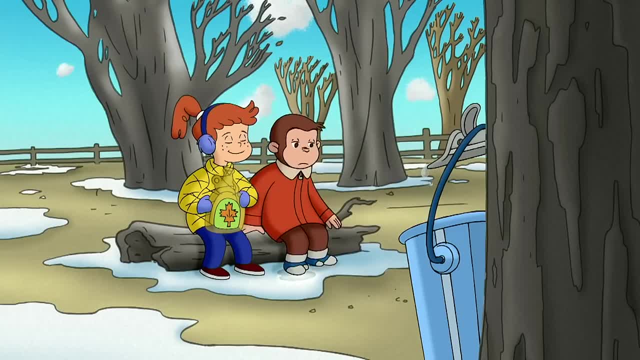 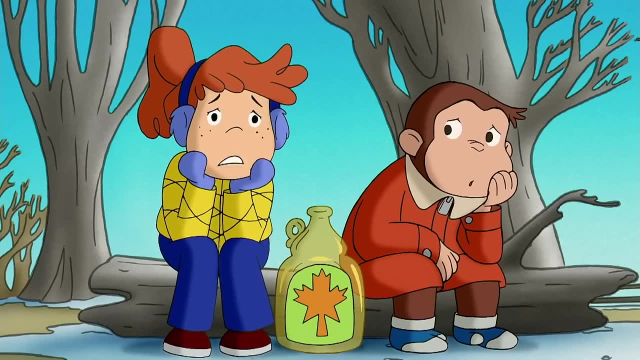 And then, when you become a good tree, you'll be able to do your job better. Y'all know that, right? Yeah, That's pretty cool. I think we tapped the slowest tree in the woods. Uh-huh, Thanks, George. 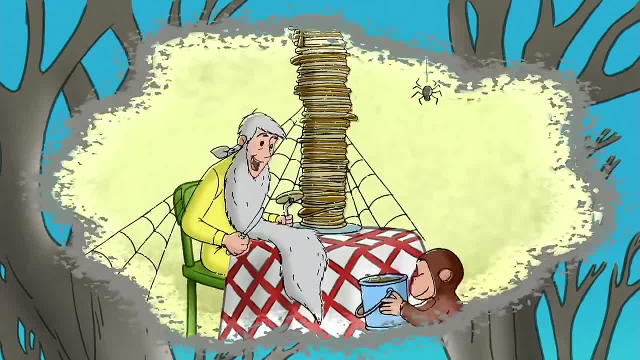 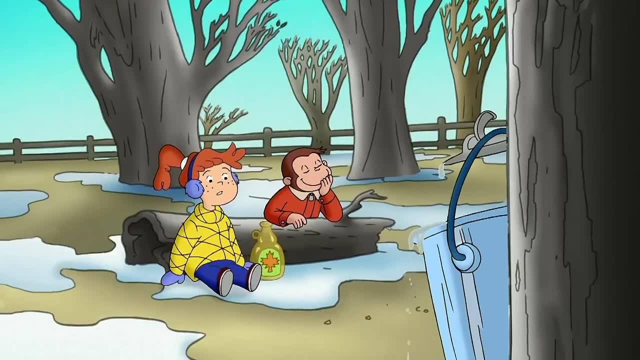 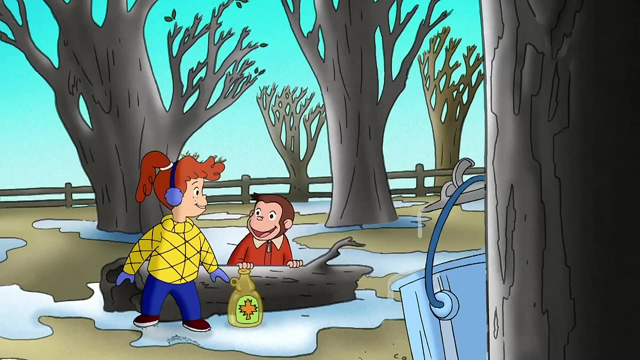 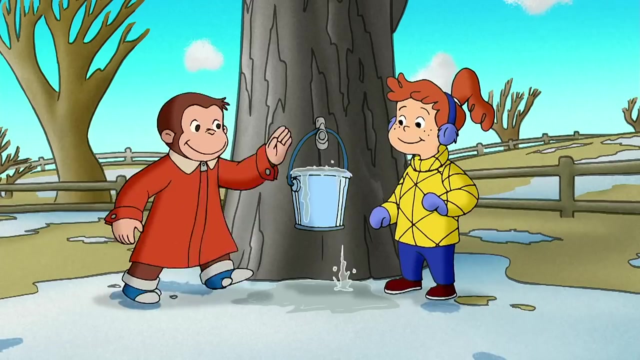 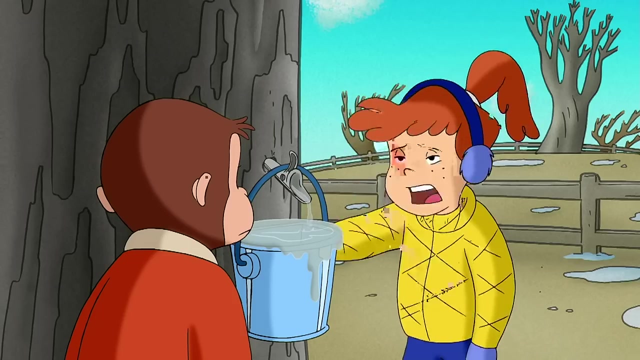 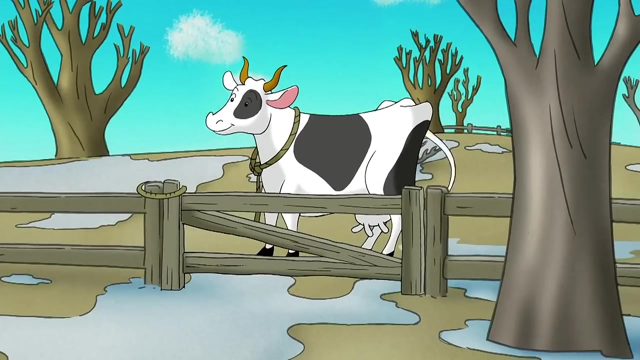 Hey George, It took a while, but George's bucket was full. Whoops, wait, I'll help you. Huh, We need a bucket lifting machine Or an elevator. Whoaa Or a cow, Yep and syrup, And we made it. 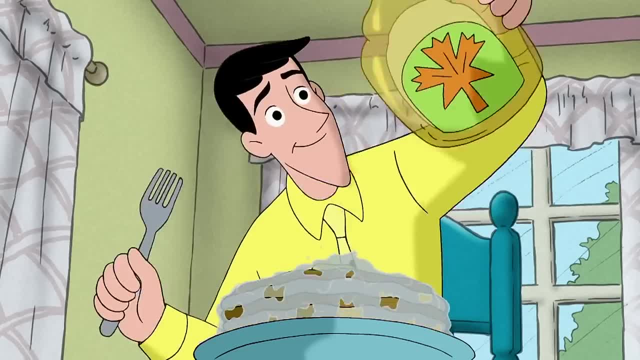 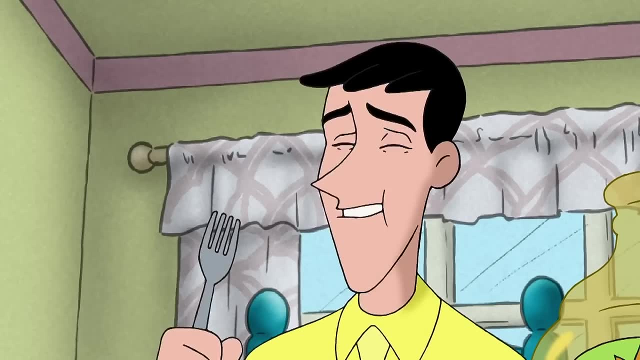 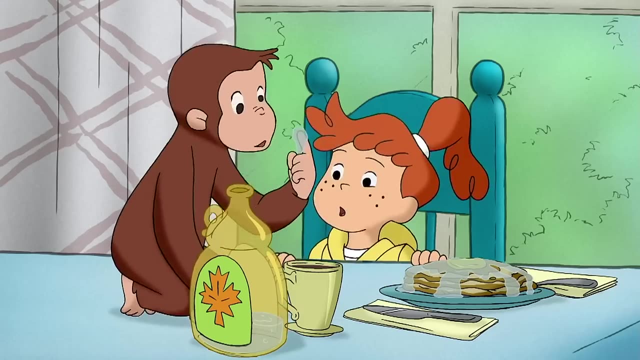 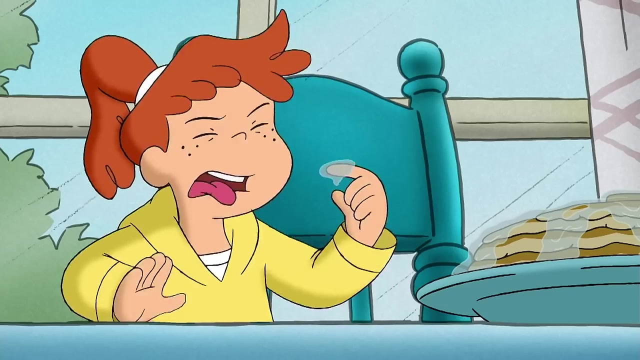 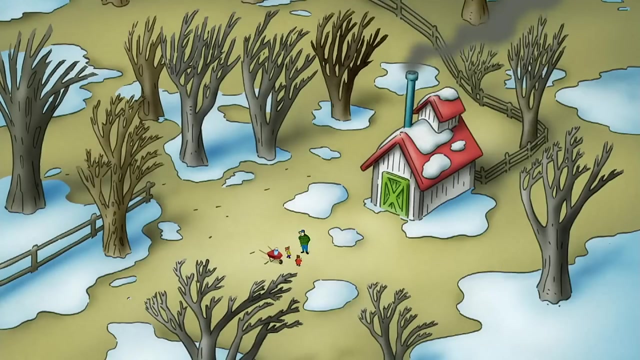 Well, the tree made it, but we tapped the tree all by ourselves. Wow, Very moist. That doesn't taste like syrup at all. Grandpa's trees must be broken. No, no, no, The trees aren't broken, George. 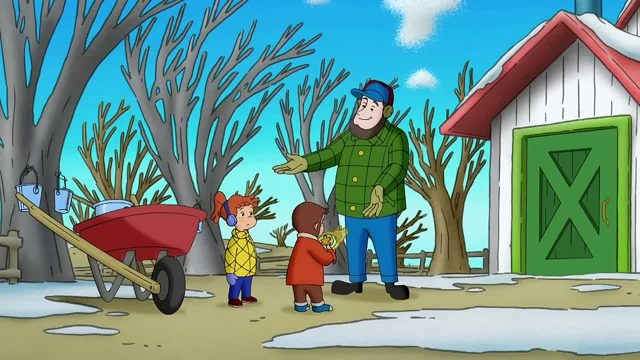 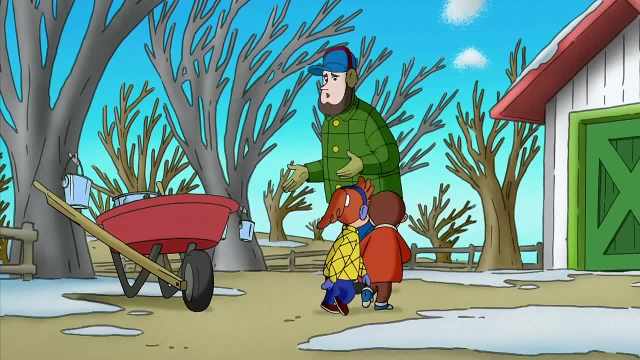 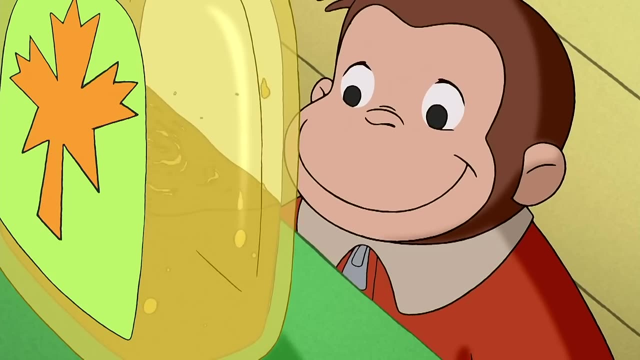 Maple syrup trees give sap, not syrup Sap. Sap becomes syrup after it's boiled down. Luckily, you've come to the right place. We boil it right here at the sugar shack. Well, here we go. Here you are your own bottle of syrup. 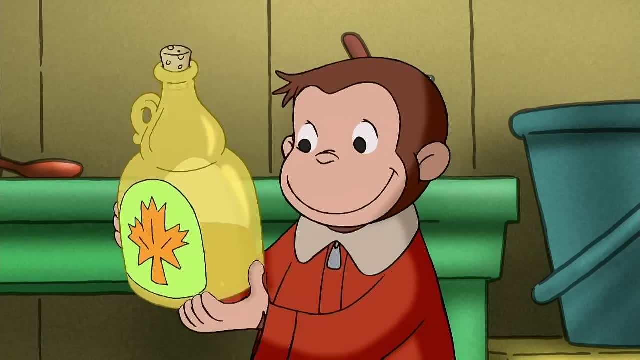 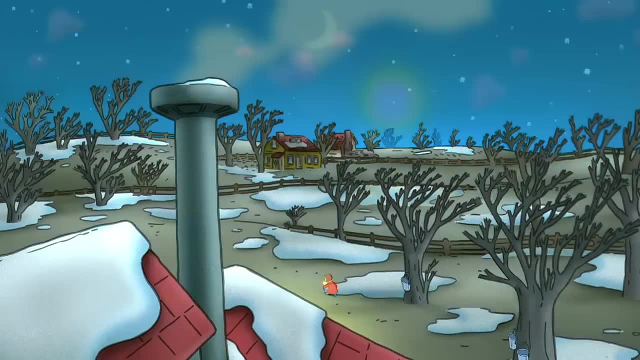 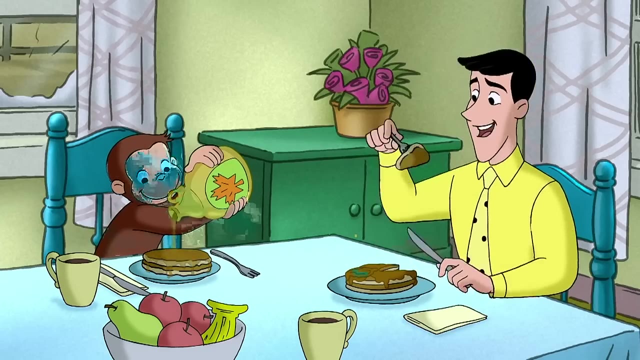 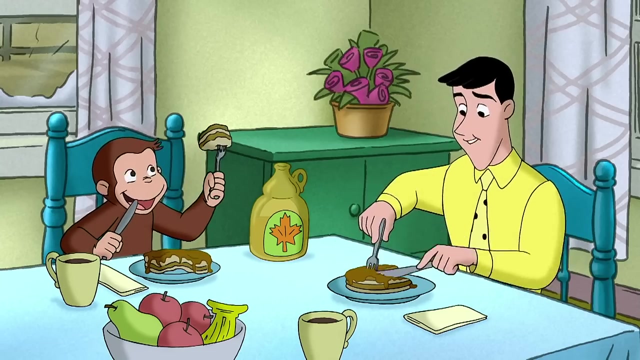 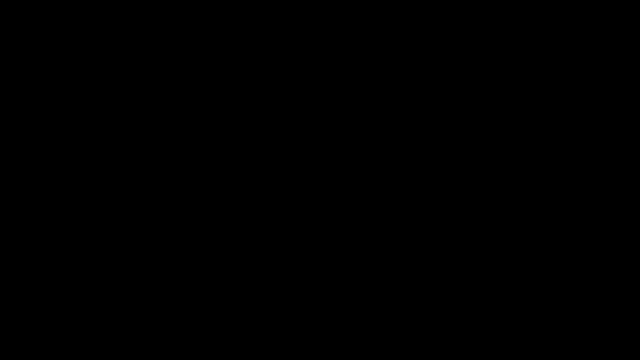 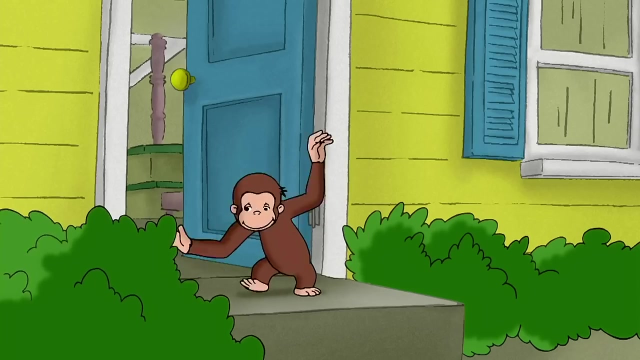 It takes a whole lot of sap to make a little bit of syrup. Uh-huh, Bye-bye. Thanks, George, Best syrup ever. Luckily, a little bit of syrup has a whole lot of taste. Most mornings George went out on the porch to find the paper. 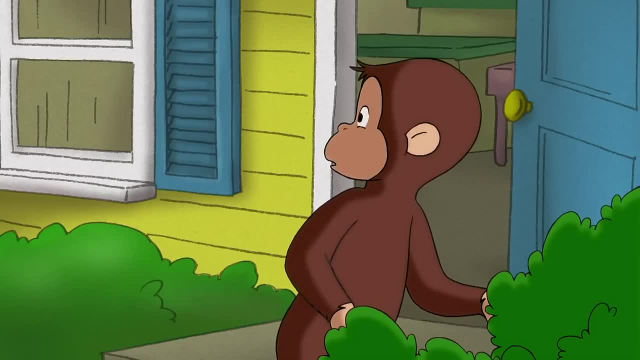 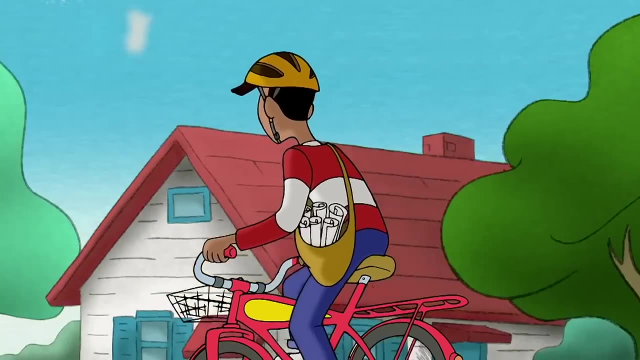 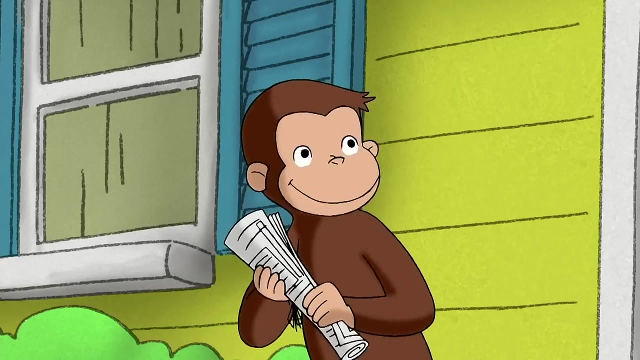 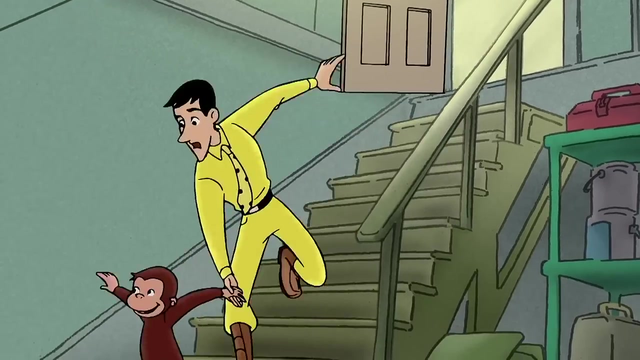 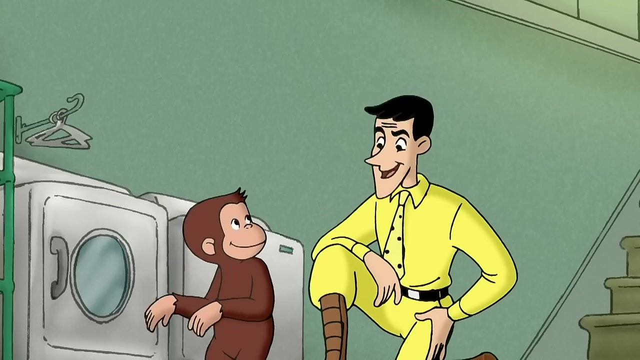 This morning the paper found George. Sorry. Oh, George wished he could be a paper boy someday, Hmm, But he didn't even know how to ride a bike, Not yet, anyway. This Why? this was my bike when I was a boy. 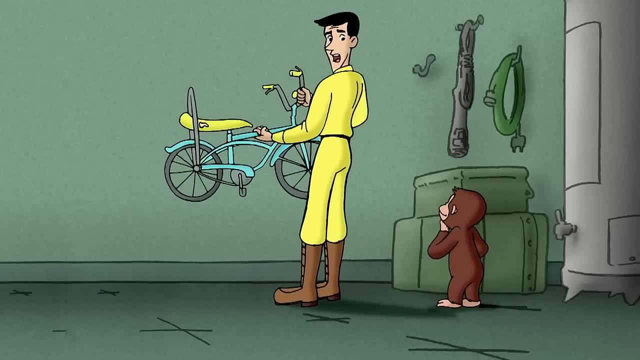 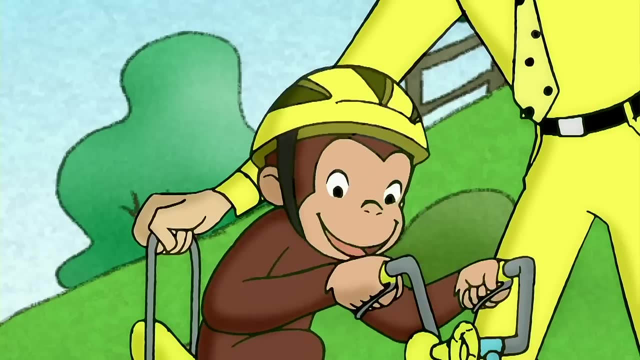 I sure had fun, But it was a long time ago. Ooh What, Oh, I remember I knew how to ride. I knew it. I know how to ride, I knew how to- I-I didn't know how to ride. 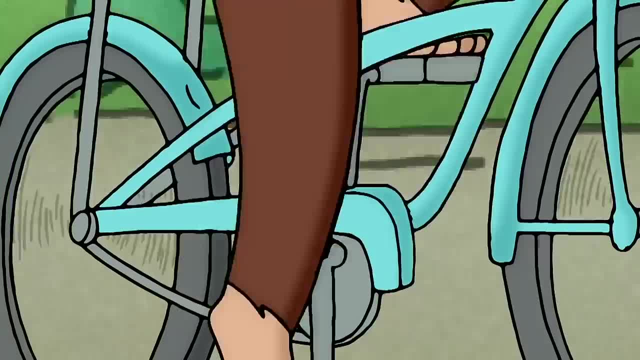 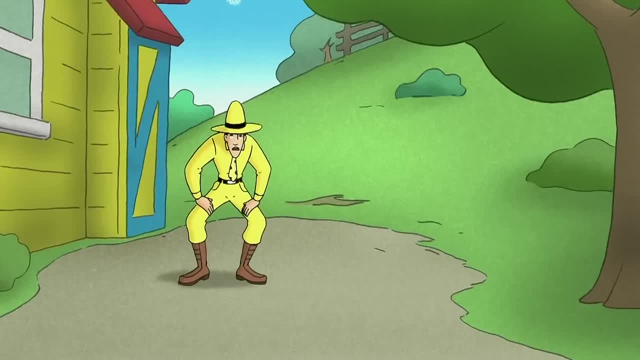 I only knew how to ride, And I knew it was your broken heart. You didn't even know how to ride. You were scared to go home, were you? But then I knew how to ride And that made me happy. I got to the airport. 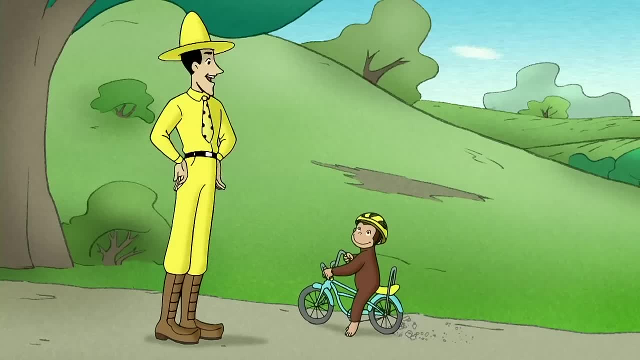 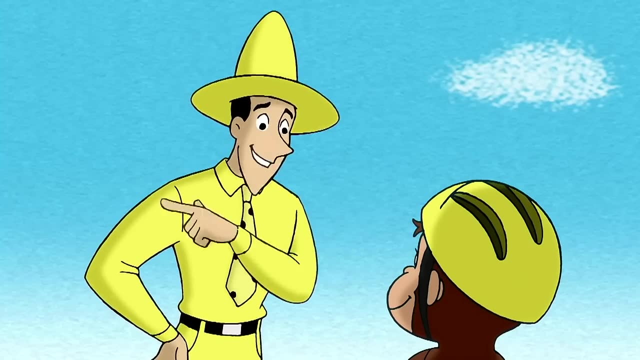 I knew how to ride. I knew how to ride. I knew how to ride You do, ready to ride on the road. now remember: always watch where you're going, stay on the right side of the road and signal turns like this for left and this for. 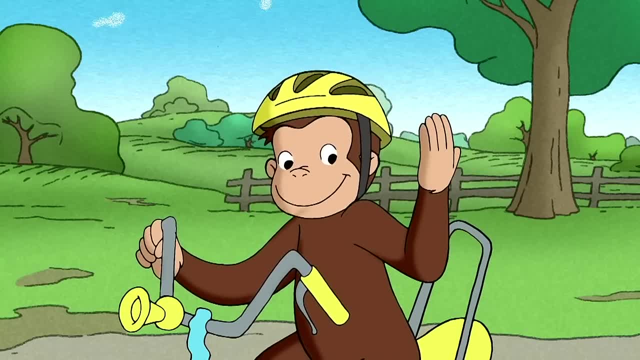 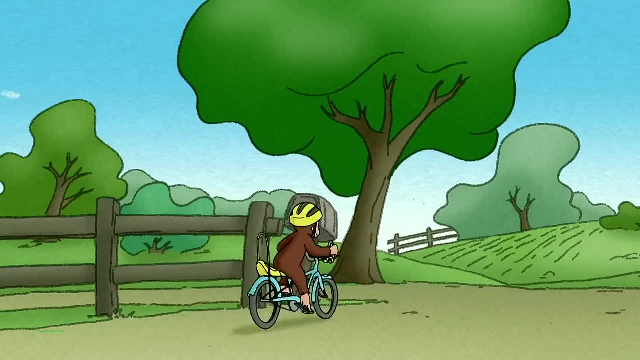 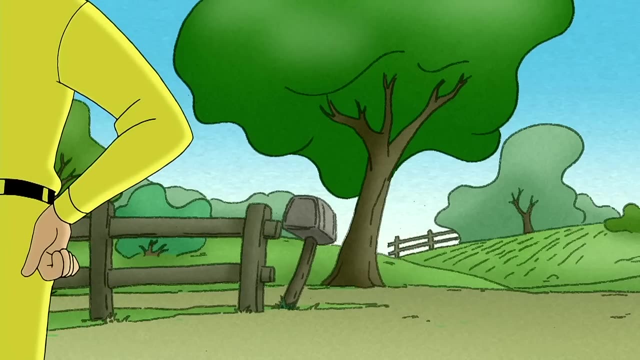 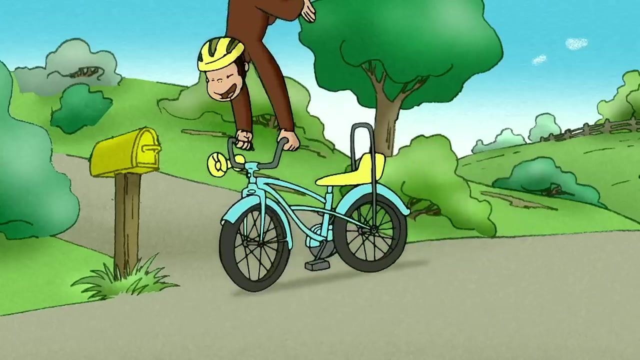 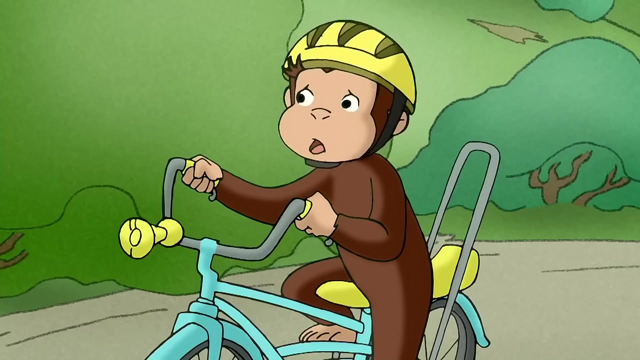 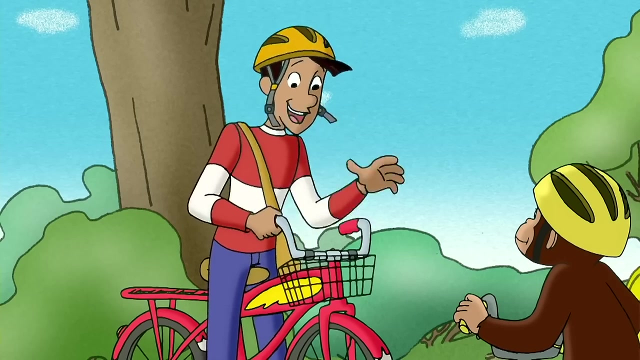 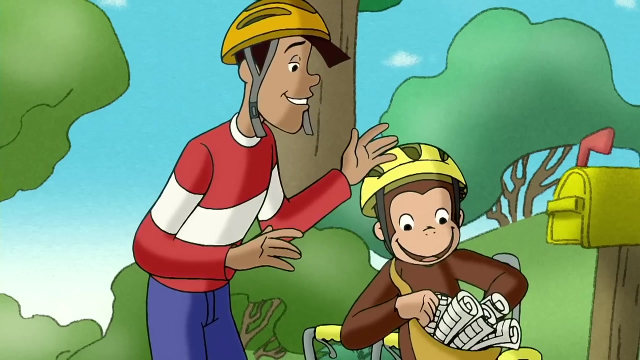 right, that's it. oh, and be a good little monkey cyclist. bye, bye. Wow, great trick. sorry I came out so fast but I'm gonna be late for school. hey, could you finish my paper out? trusted with a paper route, it was like George's wish had just come true. 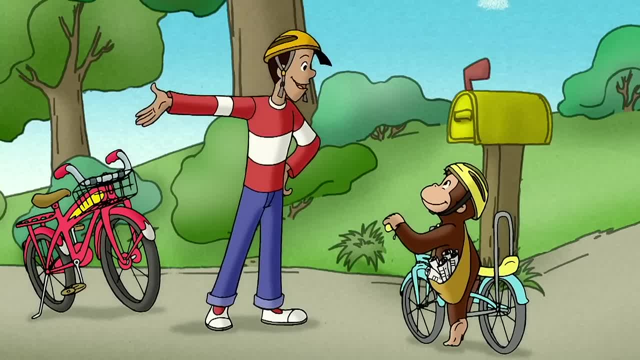 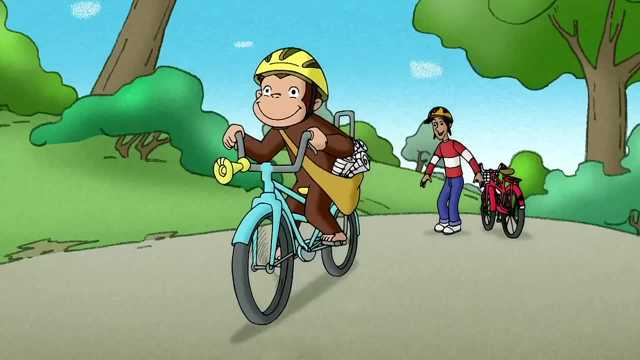 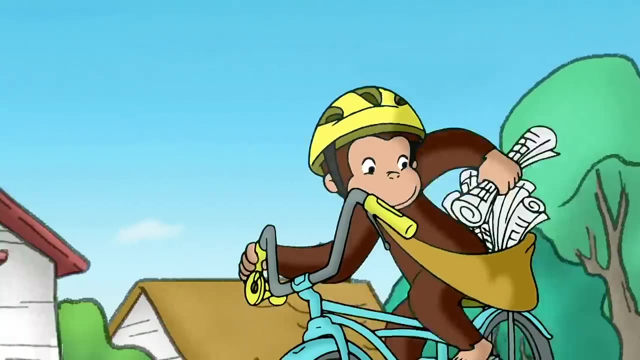 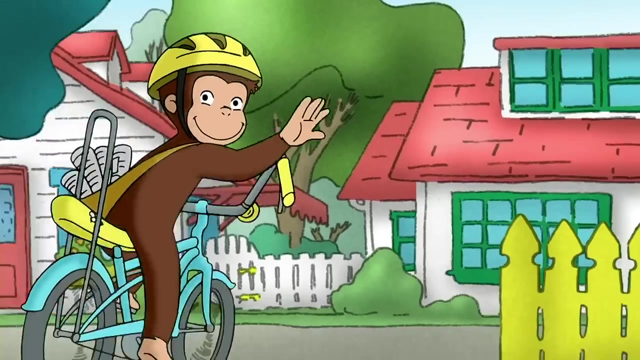 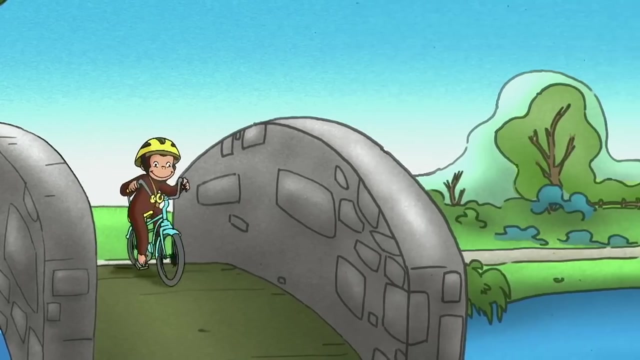 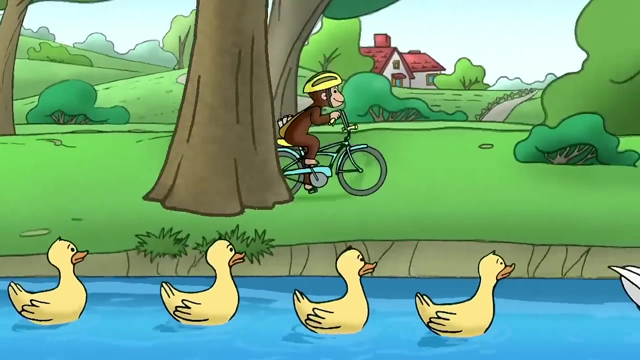 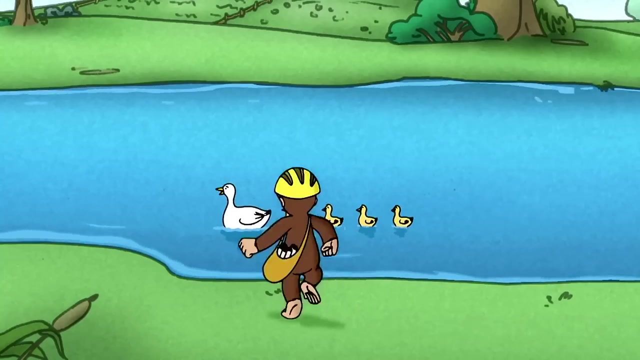 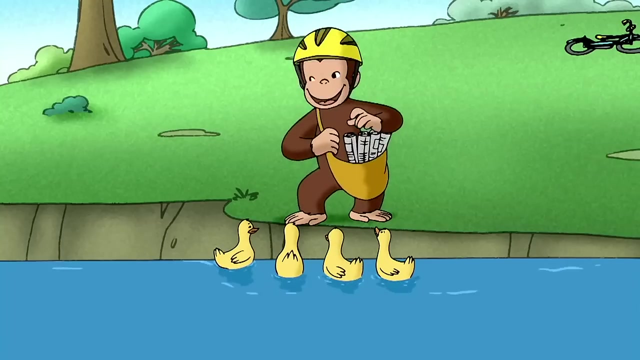 just been granted. every house on the road gets a paper, including the houses across the street. yes, George had become just like a real paper boy. nothing would stop him from completing his route. the last time they came to the stream, the man with the yellow hat made paper boats. George thought he remembered. 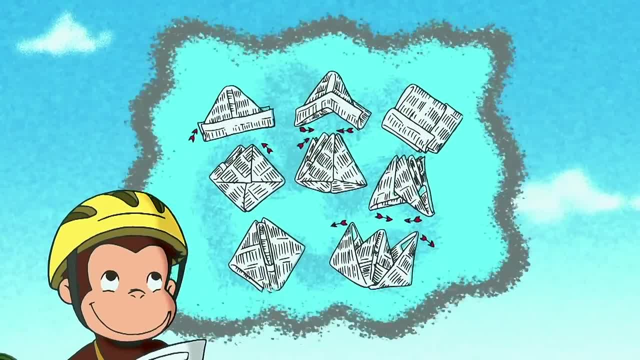 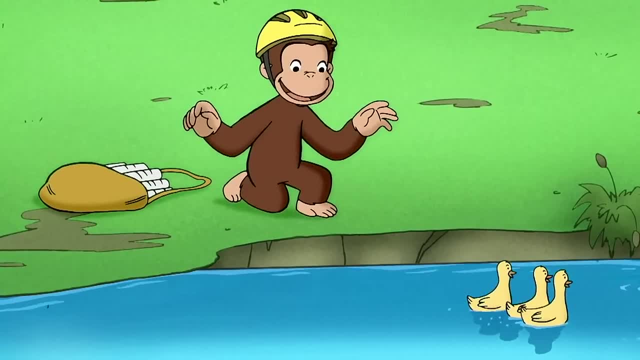 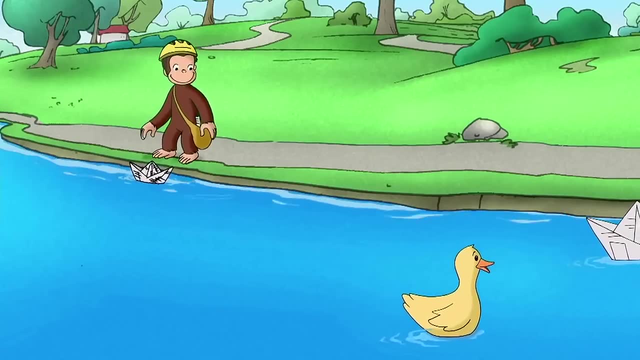 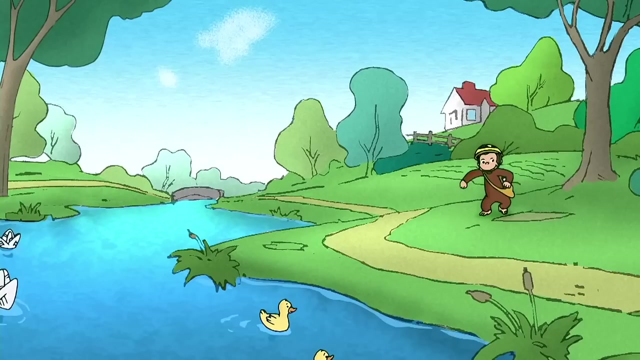 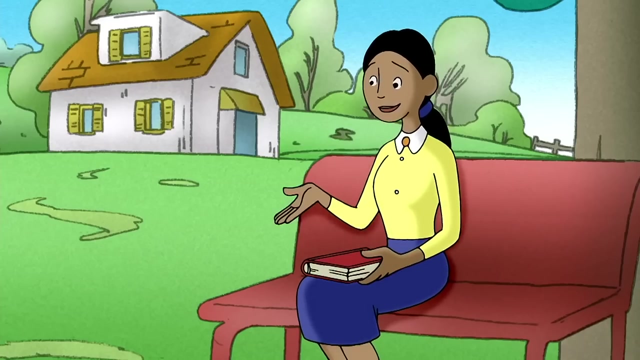 how to turn thenoria態 into a boat, But he remembered how His boat was so good. George decided to make a whole fleet. Well, hello, You must be a paper boy. That's an important job. Looks like you've delivered them all but one. 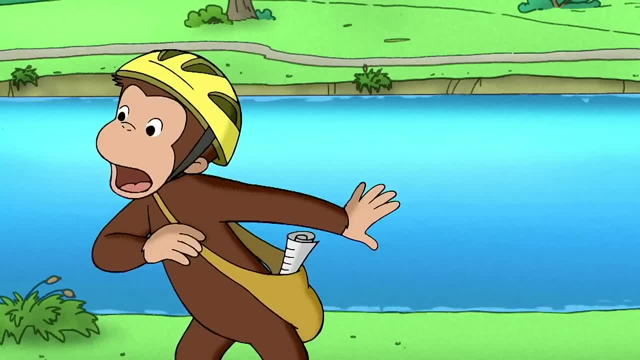 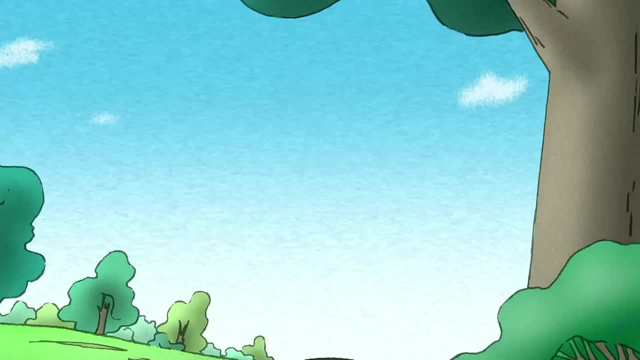 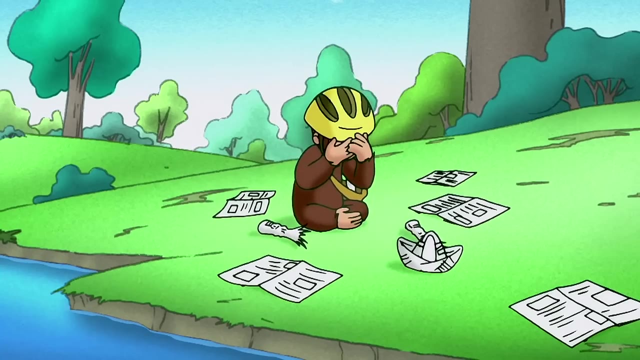 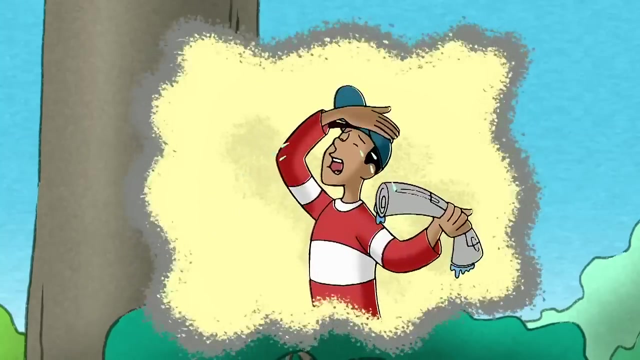 Another day's hard work almost done. eh, George couldn't wait for his newspapers to be sun-dried. George had promised Bill he'd deliver all these papers. If it didn't get done, Bill could lose his job. Maybe the man with the yellow hat knew where to get dry papers. 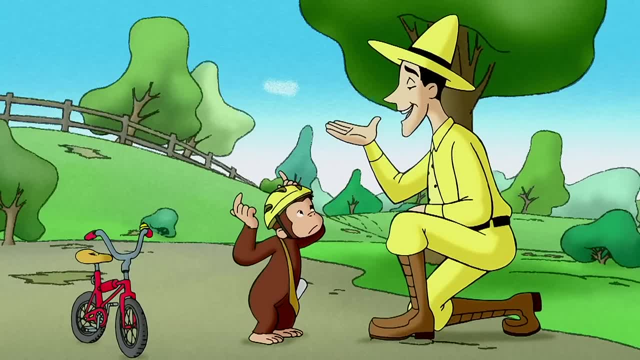 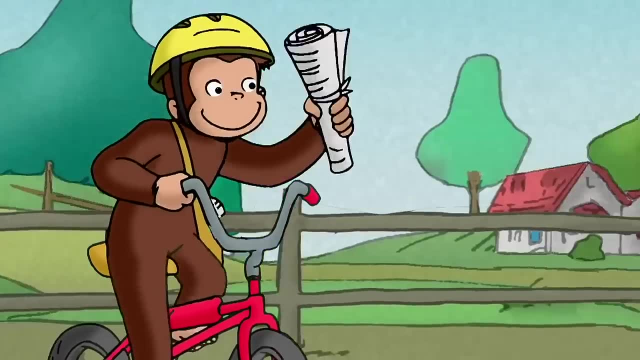 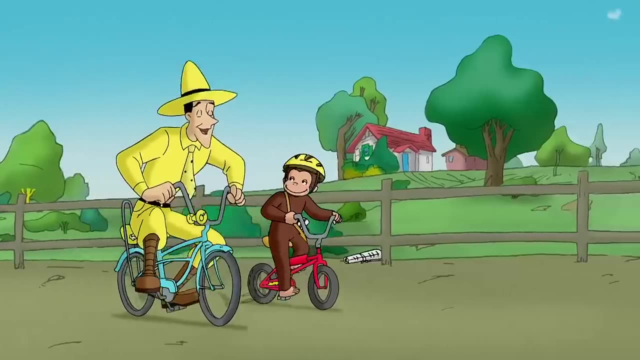 Hold on, George. How about we just buy a few dry papers and deliver them right now? And so George was able to finish his route just like a real paper boy. Maybe I should buy a new bike for myself too, Sorry. 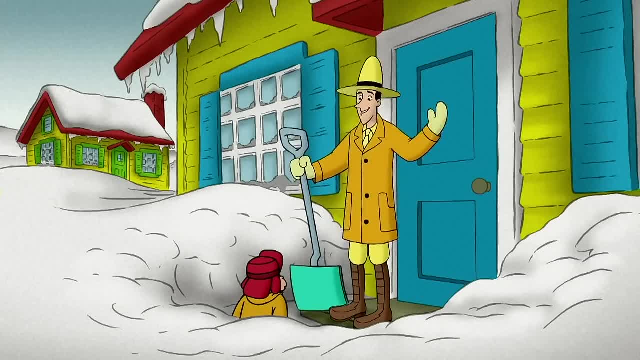 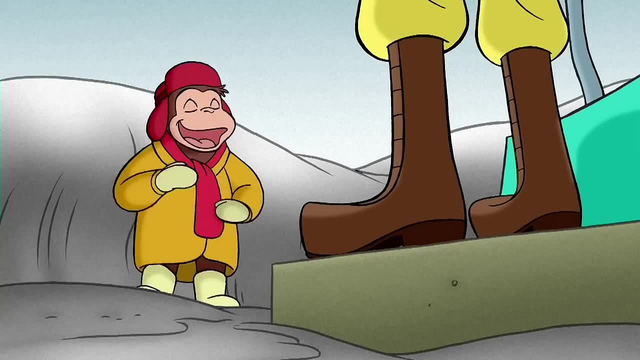 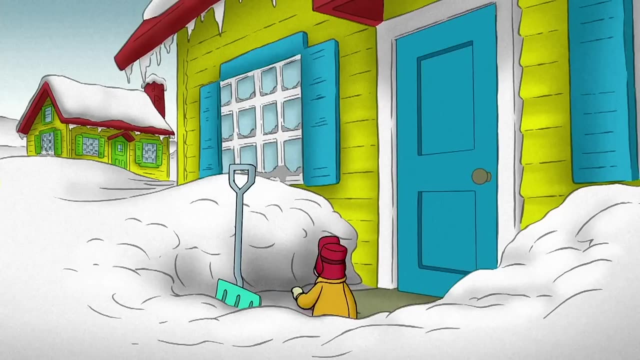 Well, I'm kind of tired, George. Hey, why don't you play while I make hot cocoa? I think we have just enough left for two cups. Playing in snow, then finishing off the good hot cocoa- This was going to be a perfect day. 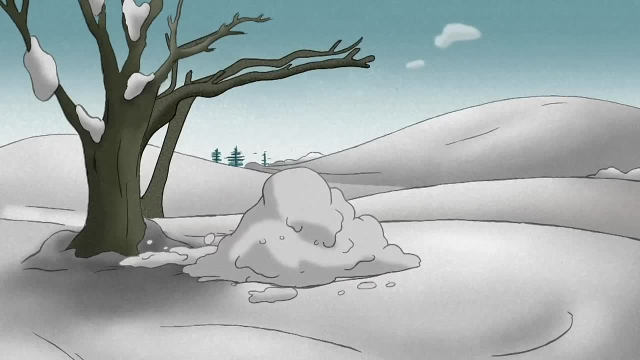 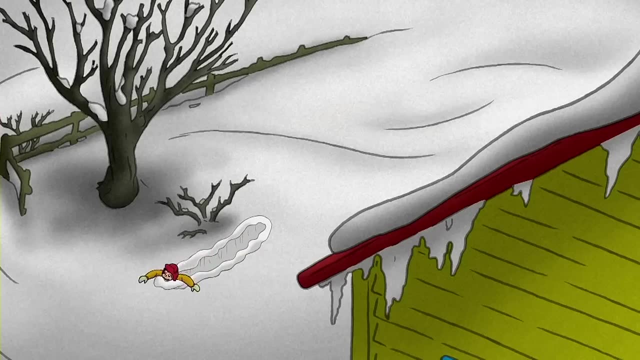 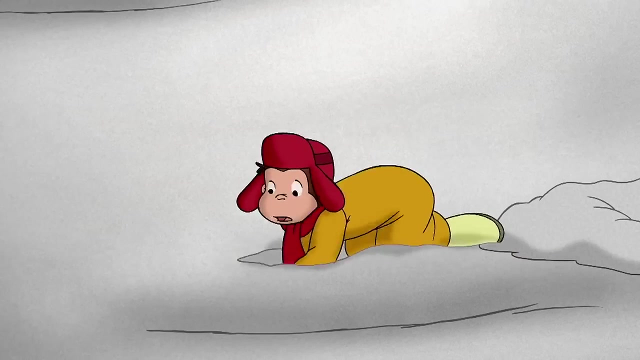 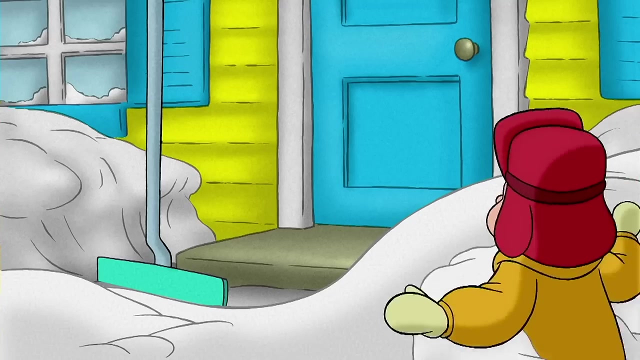 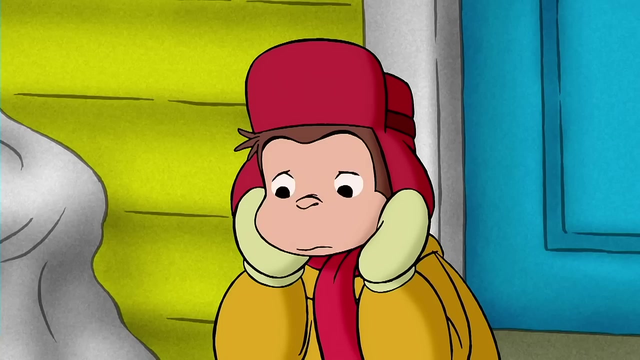 Ooh, Ah, Aw, Brr, Hey, Uh, Ha, jul, Huh, авак, Here was all this fresh snow just itching to be played with, But it was too deep for George. Hey, George, It's all mine. 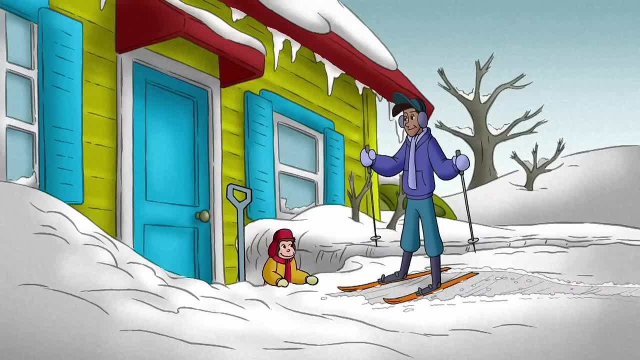 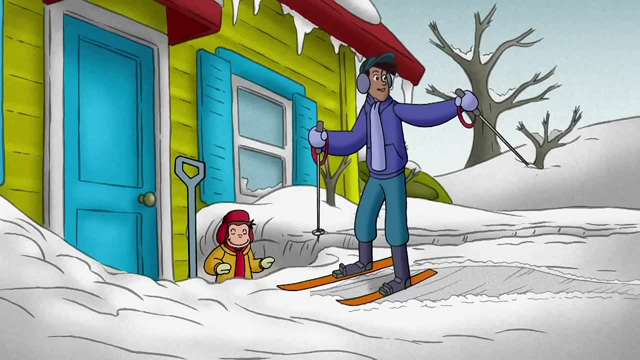 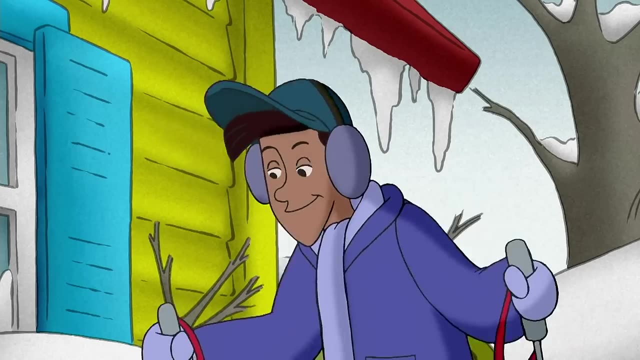 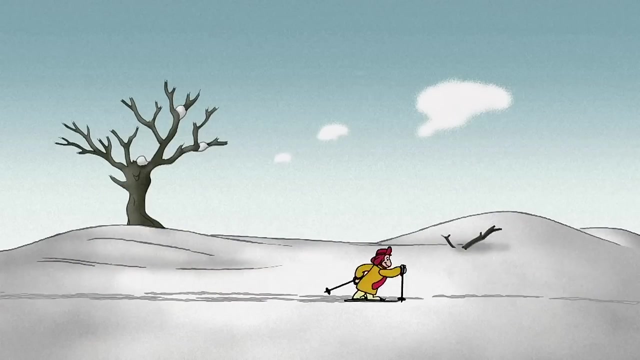 Guess the city kid wouldn't have seen cross-country skis before. It's the most fun way to travel on deep snow. I've got an old pair of skis you can have Want to come with me. This was fun. George took to skiing like a monkey to ski. 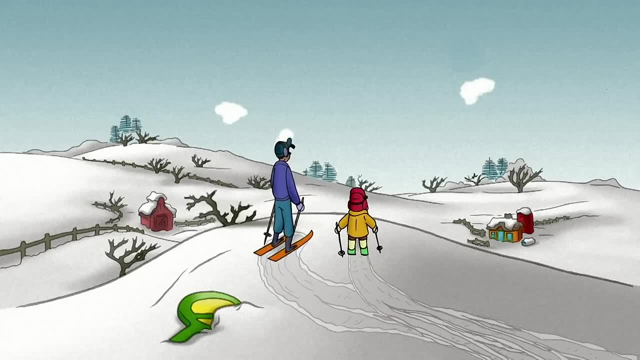 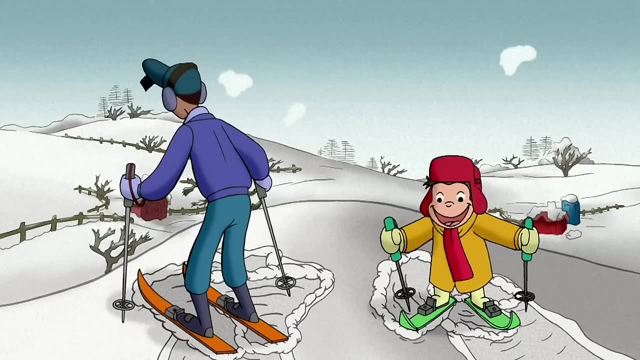 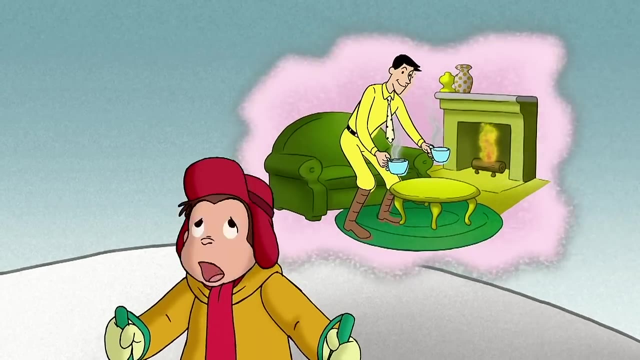 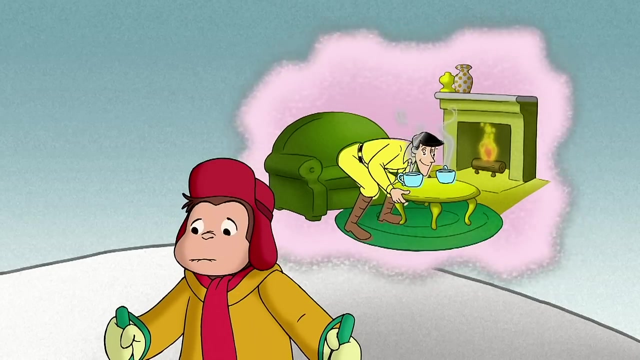 George had a great view up here. He could see houses and farms And there was his house. And then he thought he'd better head home right now, because the man was making the last of the cocoa And no one can resist the drink-me-now power of cocoa. 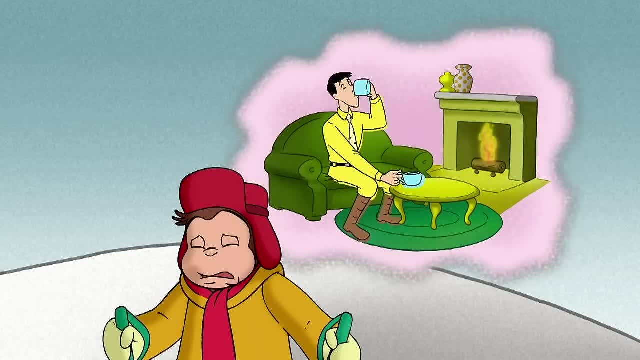 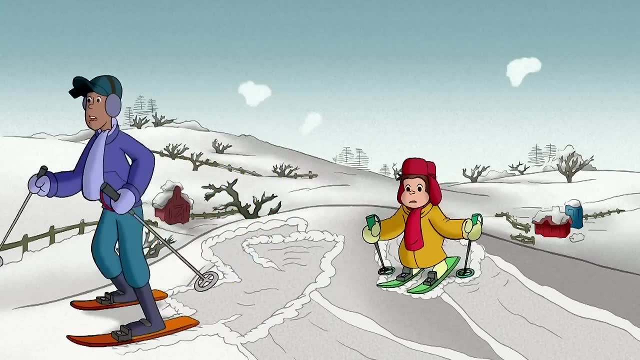 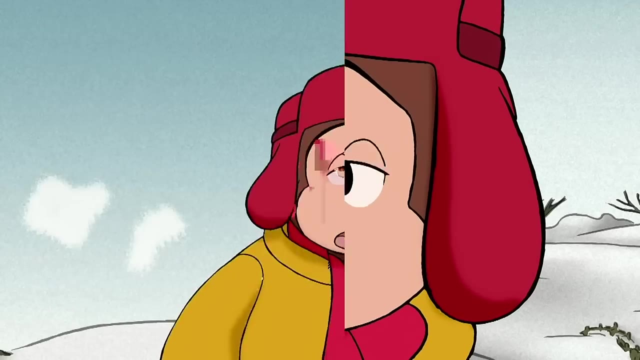 Not even the man, Not even the man with the yellow hat. I wonder what that could be. I'm going to go take a quick look around You. wait here, Hey George, Down here. I couldn't find what made that sound. 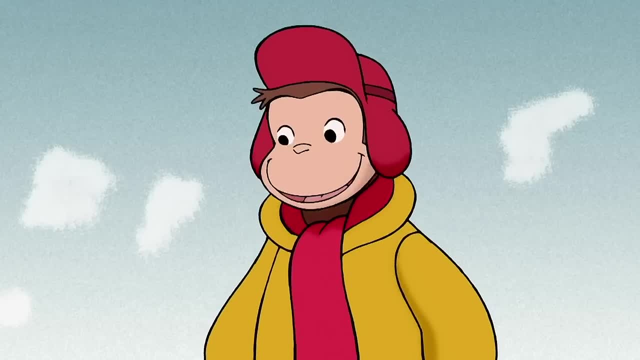 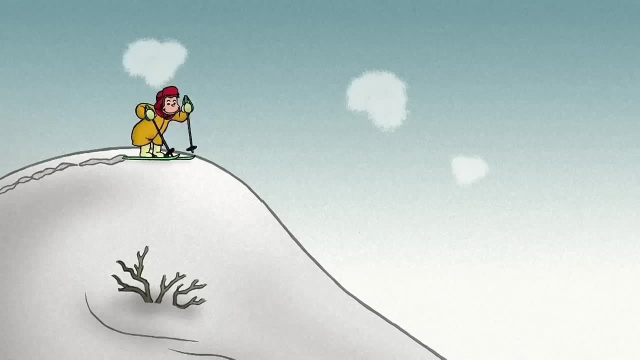 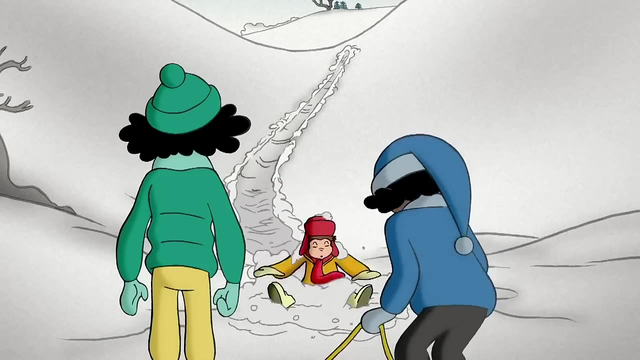 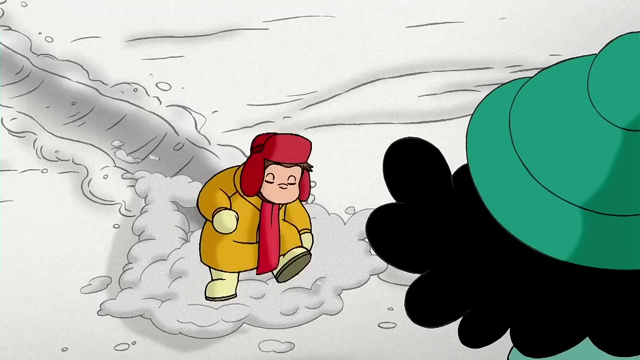 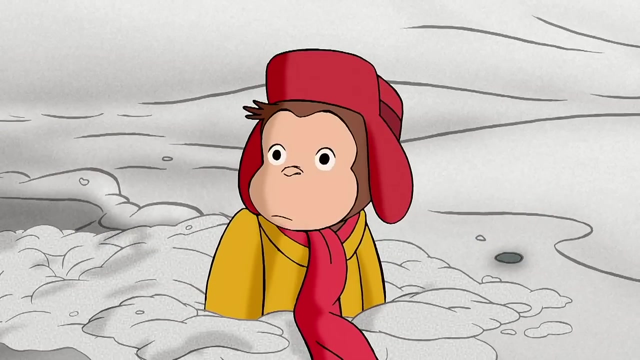 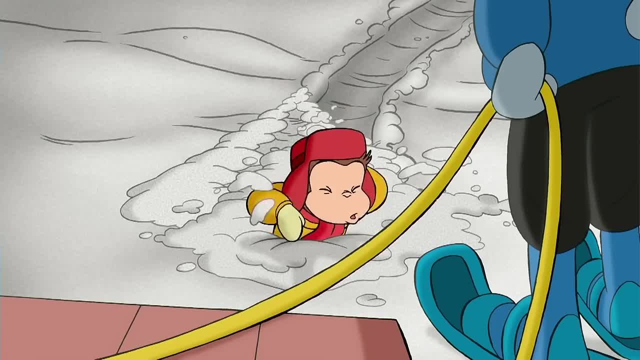 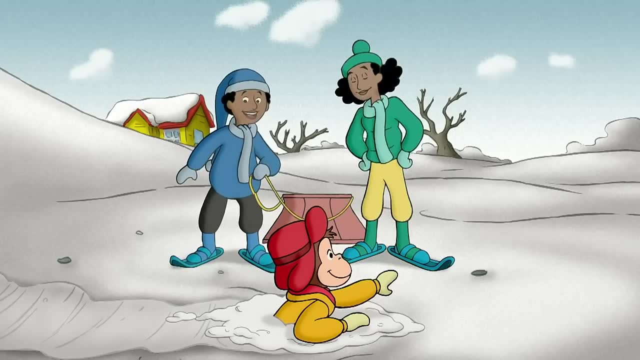 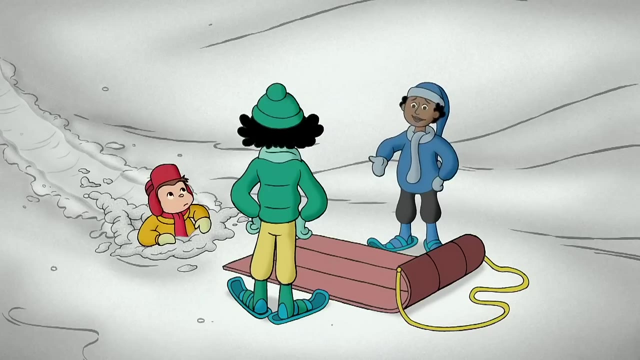 I think he likes our snowshoes. I think he wants to borrow our snowshoes to get to that house. He probably lives there. I'll give him mine. Then how do you get home? You can't walk on the snow without them. Let's pull him home on our sled. 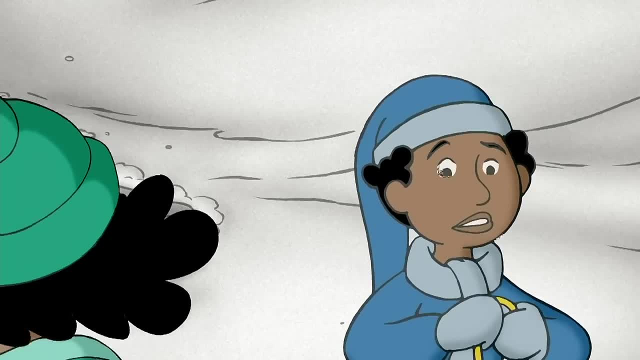 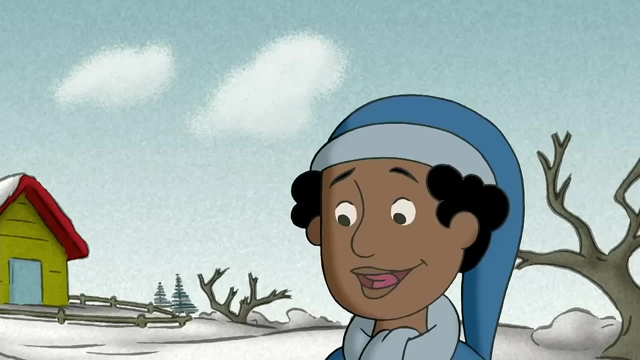 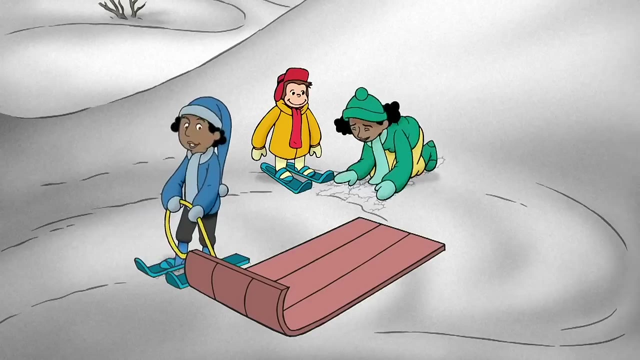 Kent, we're already late and Mom's going to get worried. We can't just leave him here. How about we get ourselves home first and then we'll give the monkey your snowshoes? We live on the other side of the hill. Climb aboard Later. 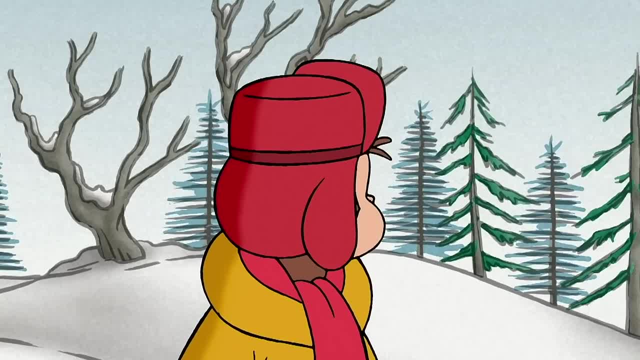 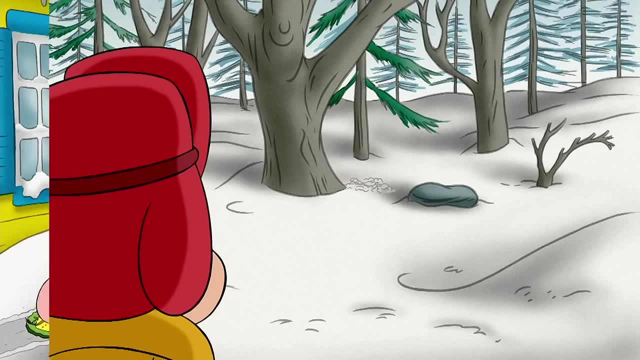 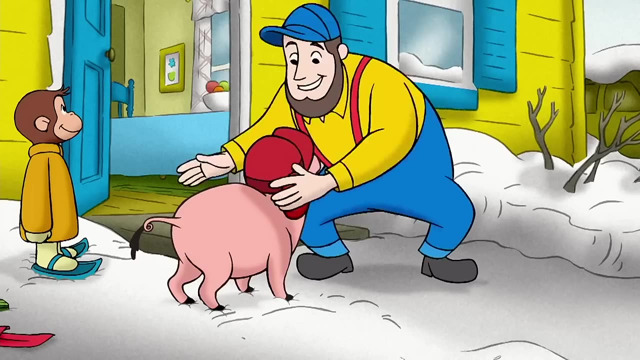 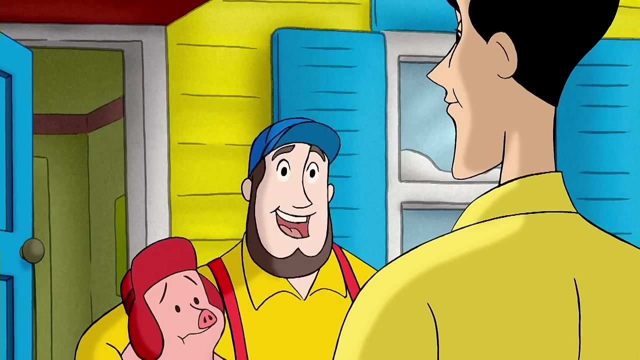 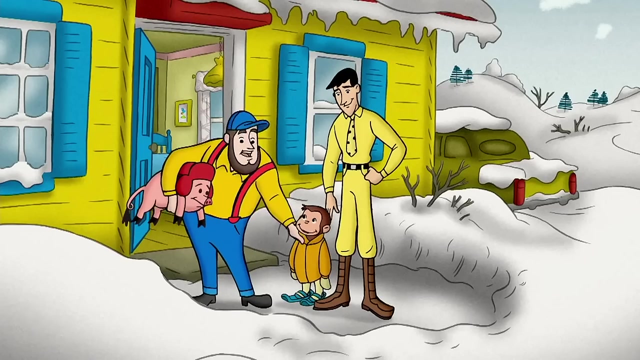 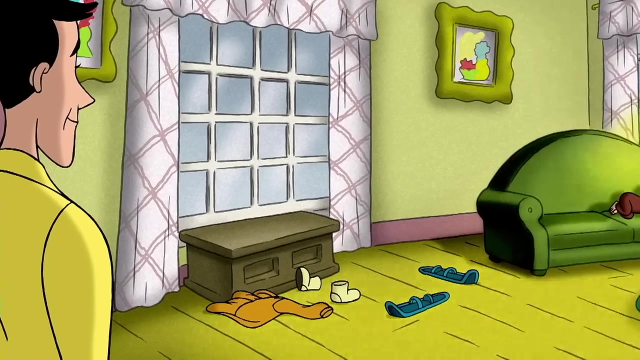 Bye, monkey, Bye. Now George could see what made that sound: A cold, lost pig. Oh, He got out last night before it snowed. He's never even seen snow before. Must have been completely mystified by it. Thank you, George, Skiing, sledding, bringing a pig home. 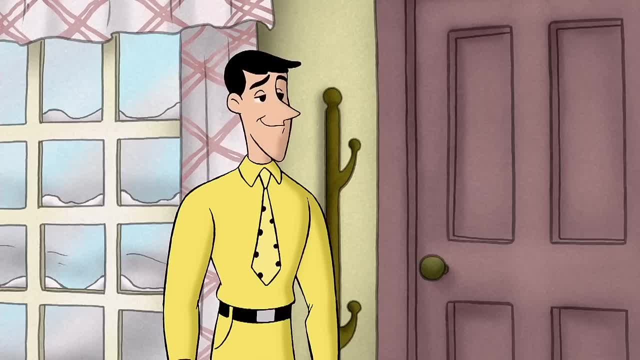 Then he got out last night before it snowed. Then he got out last night before it snowed. Then he got out last night before it snowed. Then Coco, Then Coco. This was a perfect day to be a monkey. This was a perfect day to be a monkey. 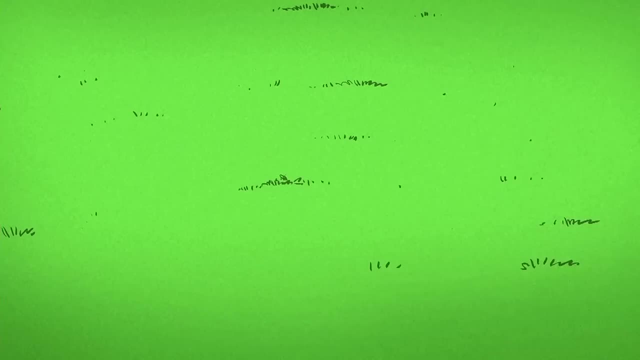 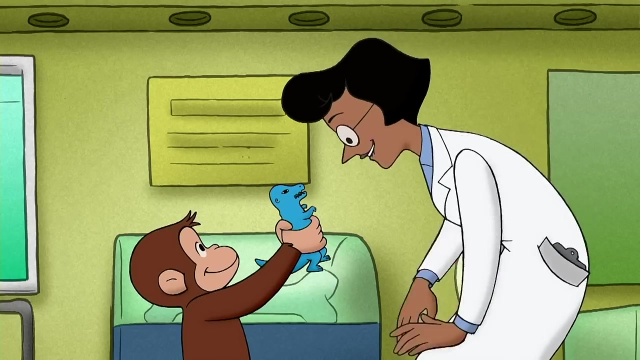 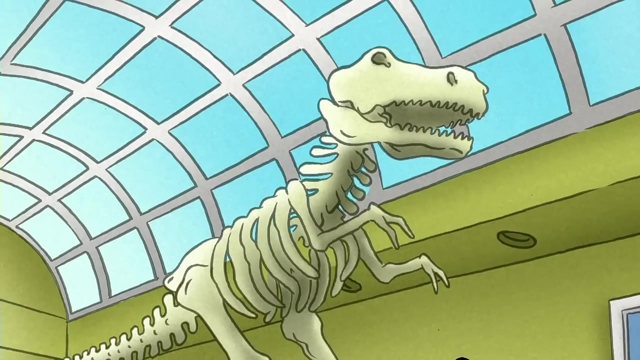 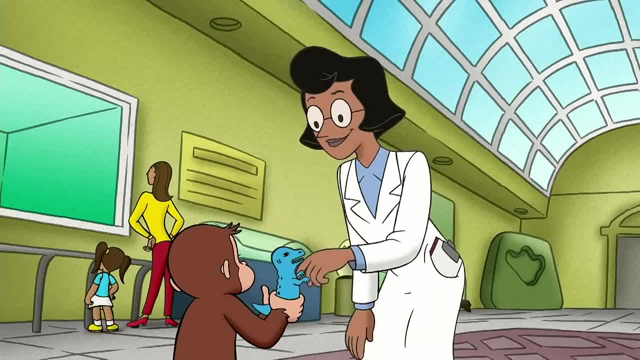 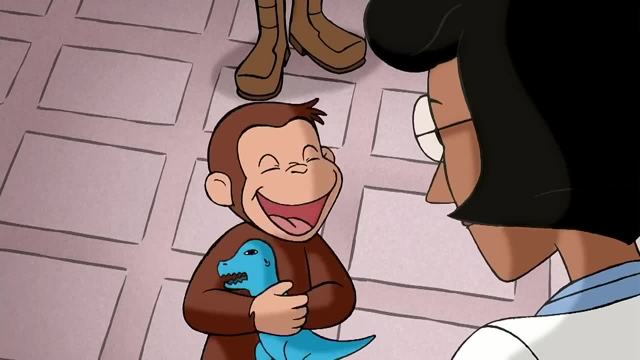 Those are the bones that would be inside that. Huh, You know, same as the bones in you. Huh, Uh-huh, Uh-huh, Uh-huh, Uh-huh. Feel your arm: The hard part, That's bone. 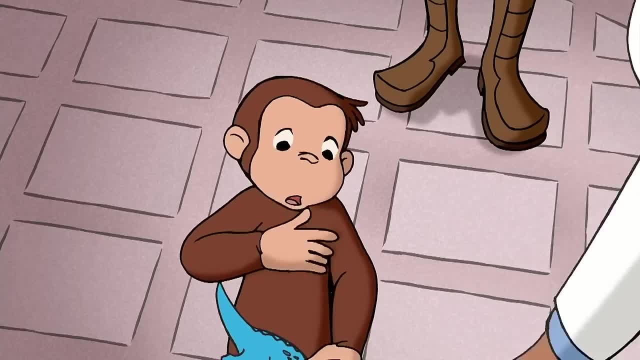 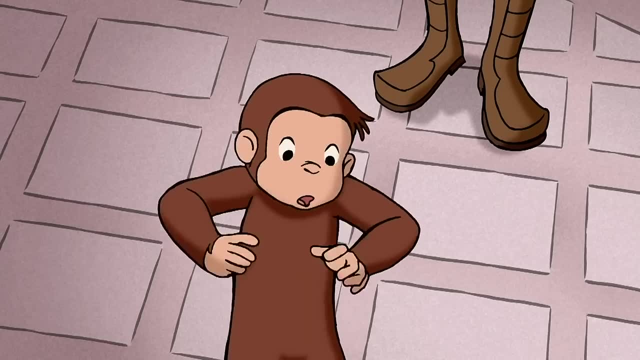 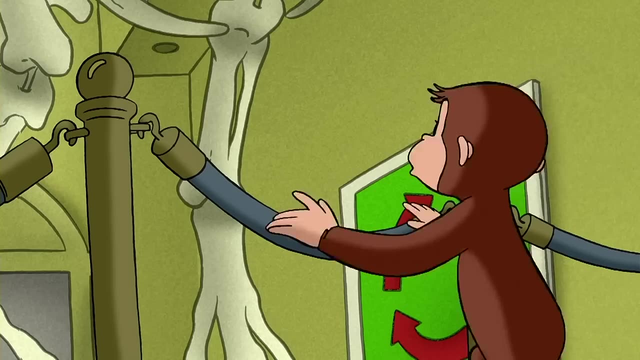 It's your skeleton. Wow, Uh-huh, Uh-huh, Uh-huh, Uh-huh. Now that he knew he had one of those under his face, George had to see the T-Rex skull up close. Woo, Ha-ha-ha. 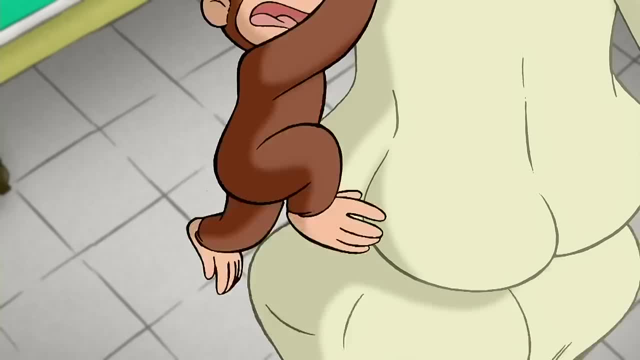 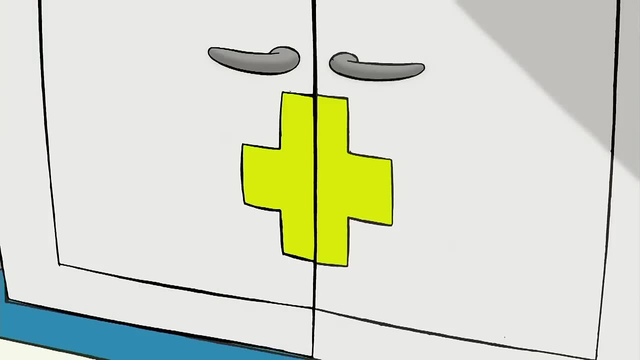 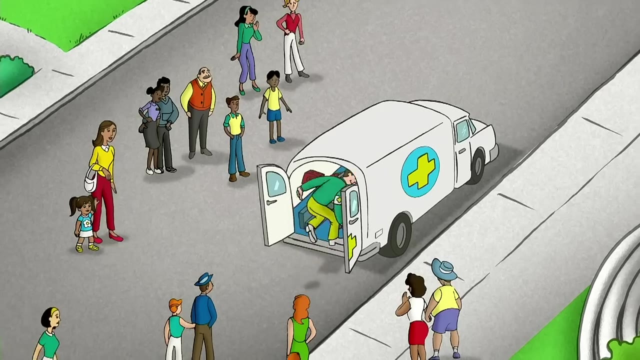 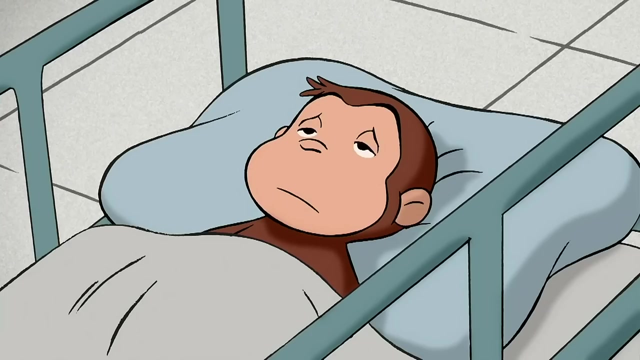 George don't, It isn't safe. Ah Ugh, Are you okay? I'm okay, Woo-hoo-hoo-hoo. George always wanted to ride in an ambulance, but he couldn't really enjoy it. At the hospital, Dr Baker decided they needed. 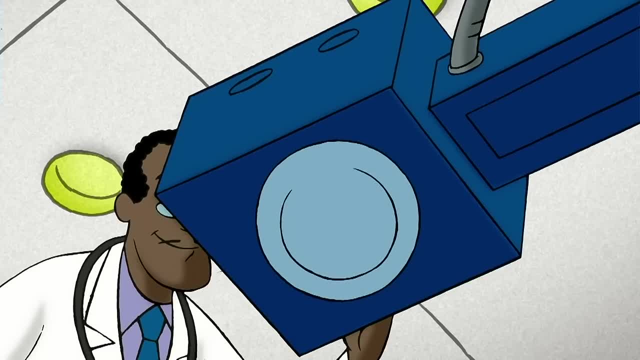 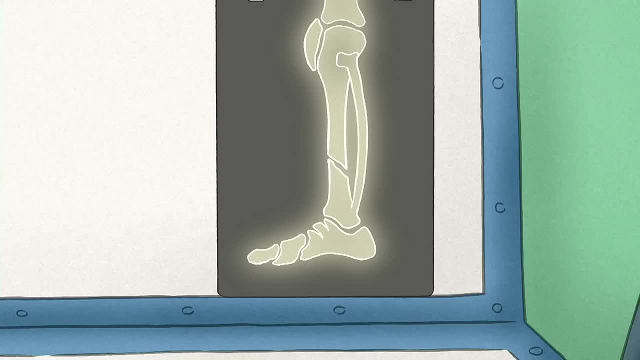 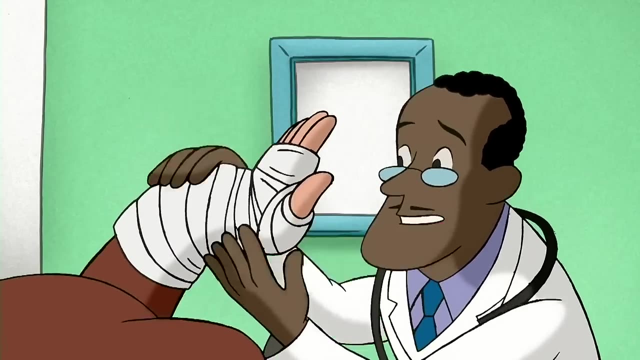 to see George's leg bone by taking an x-ray. That's a small break. We have to put your leg in a cast. Oh, Now, this cast will keep your leg from moving while the bone heals. Oh, Hey, Whoo. 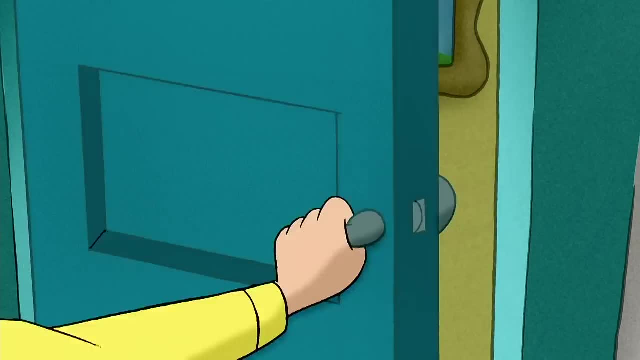 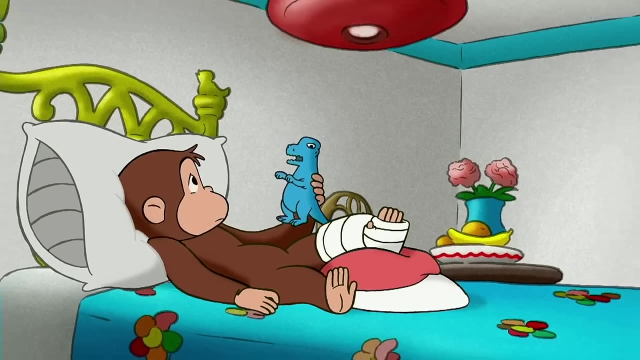 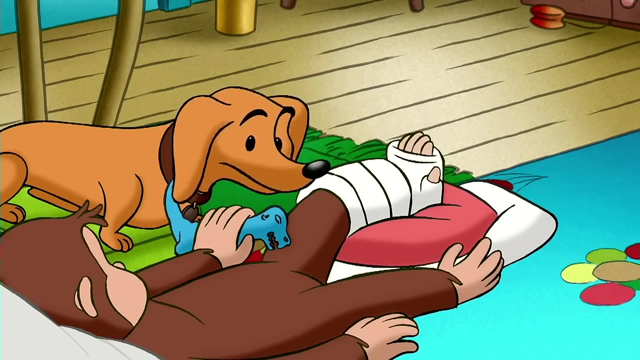 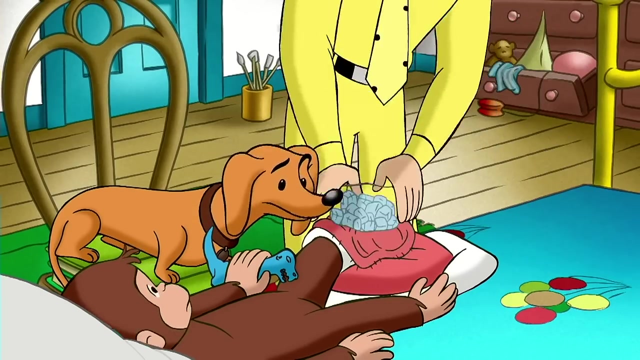 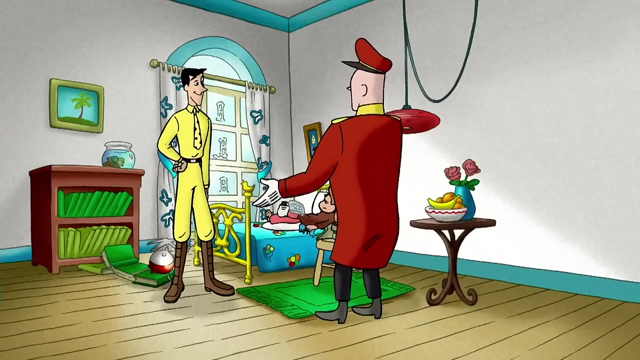 Whew, Well, hello, You have a visitor, George. It was George, all right, No one else in the building smelled like that. Hello, Hunley, come up here. Yeah, we're in George's room. You know, in the lobby Hunley pays more attention to George than anyone. 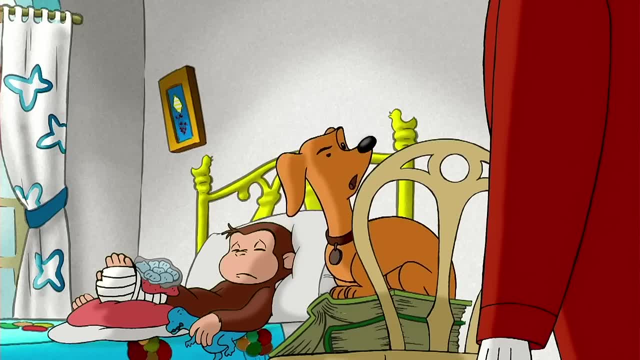 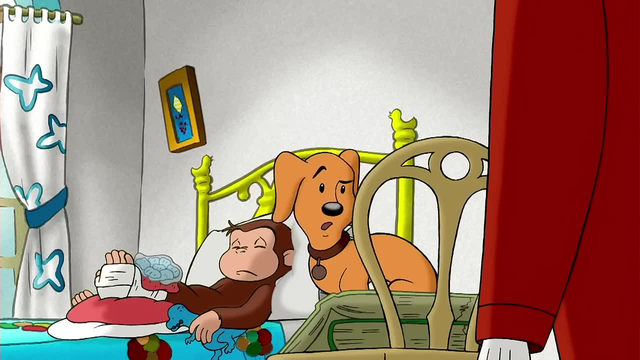 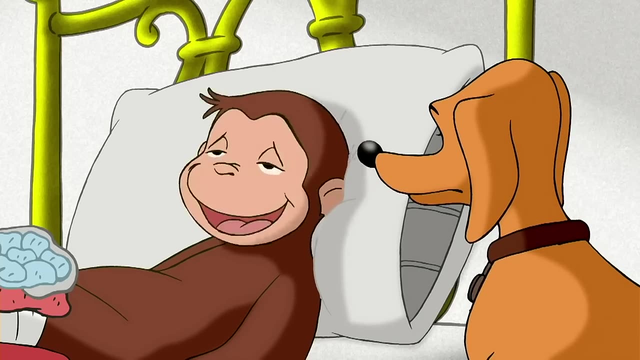 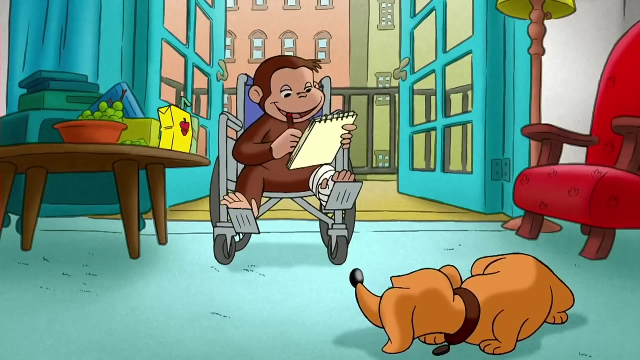 That's friendship. Hunley could keep George company when you go to work. I'd excuse him from his lobby duties. George, would you like Hunley to be your monkey sitter? Hunley was curious about this new calm. George, Ah, 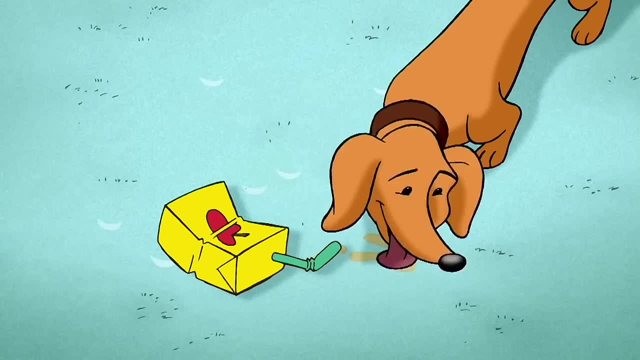 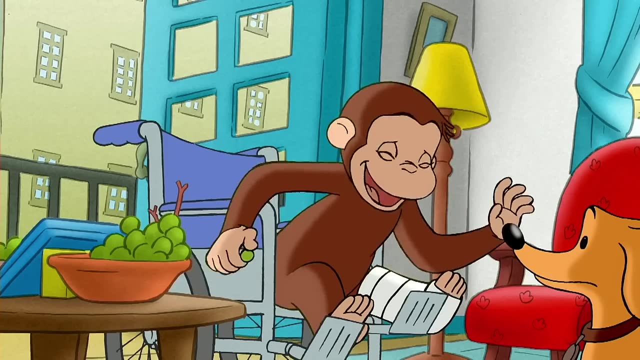 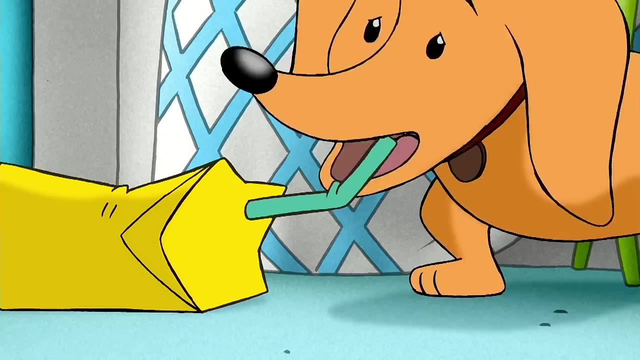 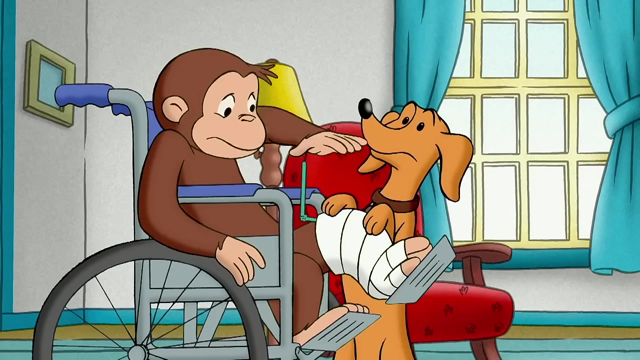 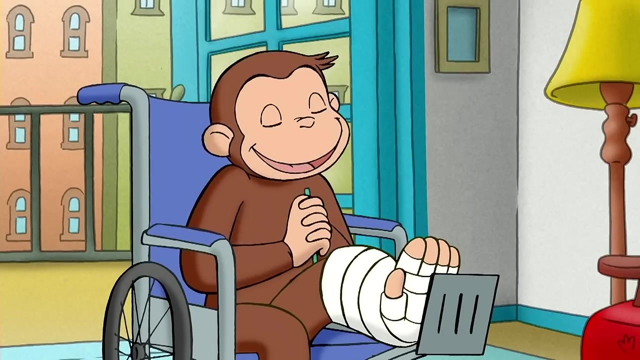 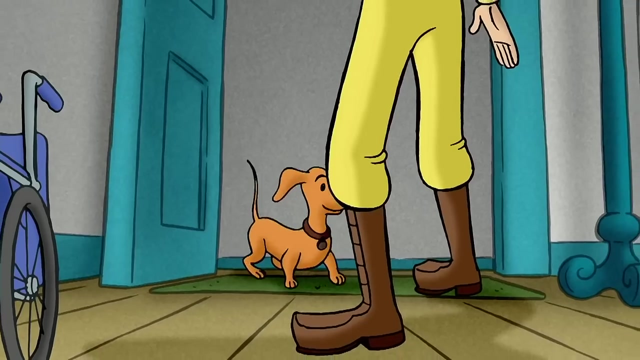 There was more to monkey-sitting George than guiding him around the furniture. Hunley cleaned up after him too, which had its rewards. He also helped with those itches that George couldn't reach. Good morning to you too, Hunley. 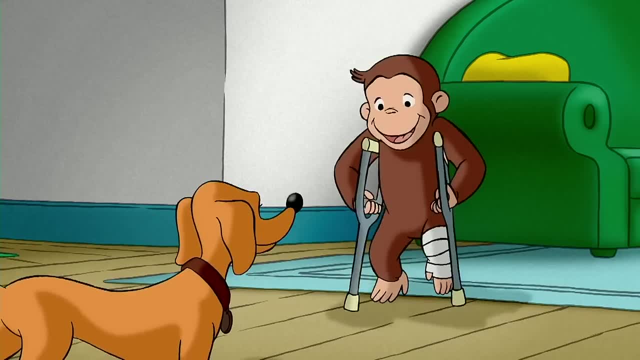 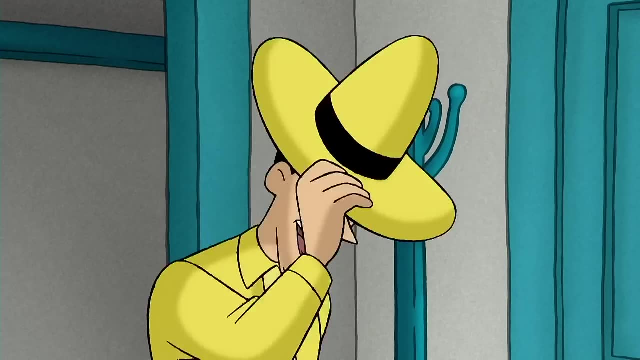 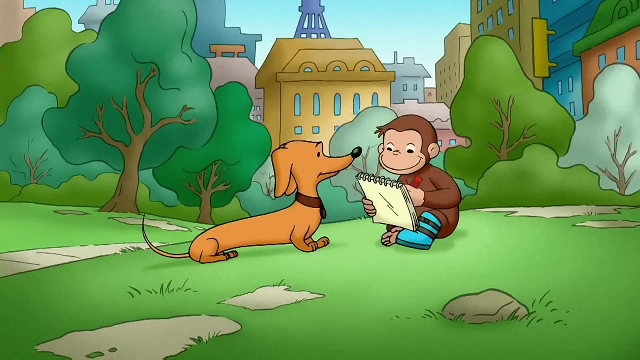 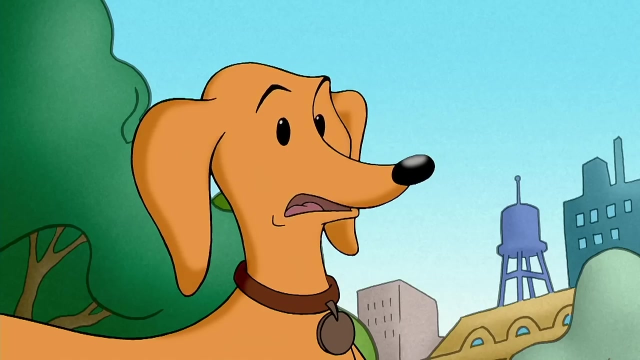 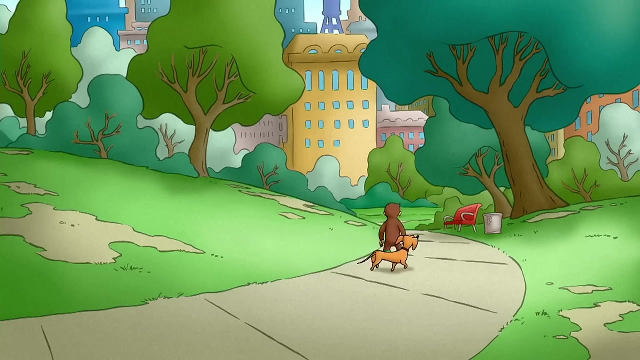 And then something changed. Remember, use the crutches, don't step on your cast and be a good little monkey. And dachshund Huh, They went to the park every day. George drew some good pictures And Hunley discovered he liked lying on grass and taking slow strolls with a monkey. 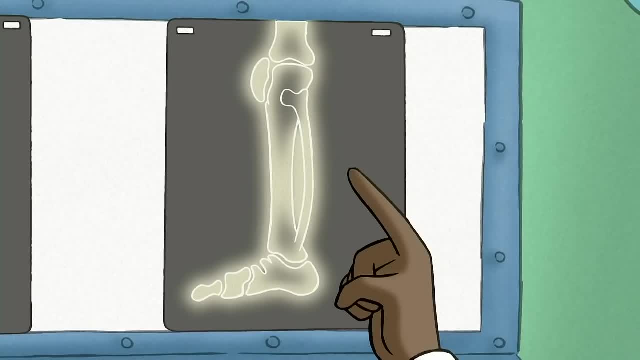 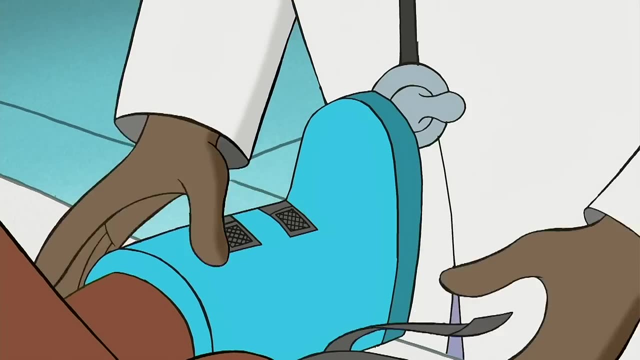 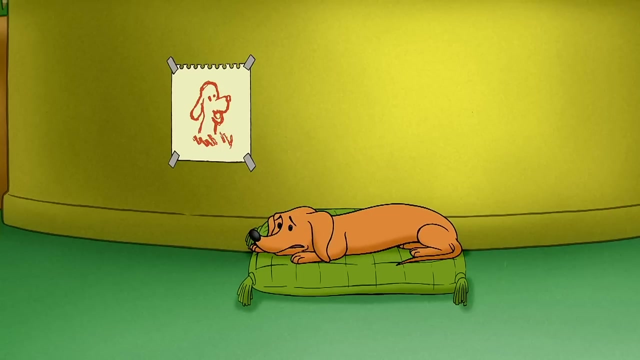 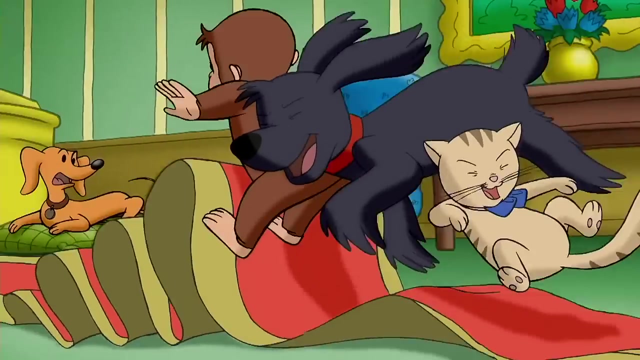 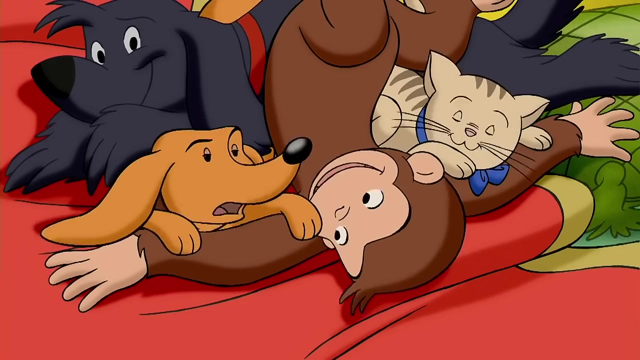 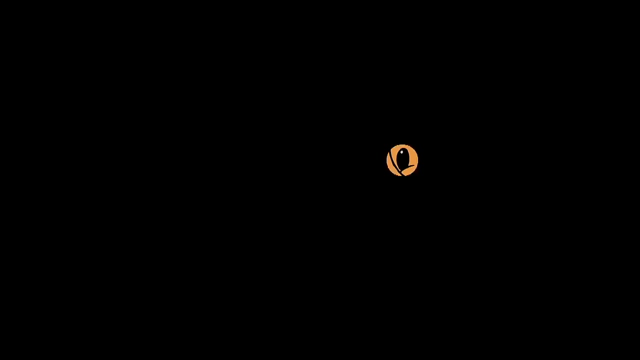 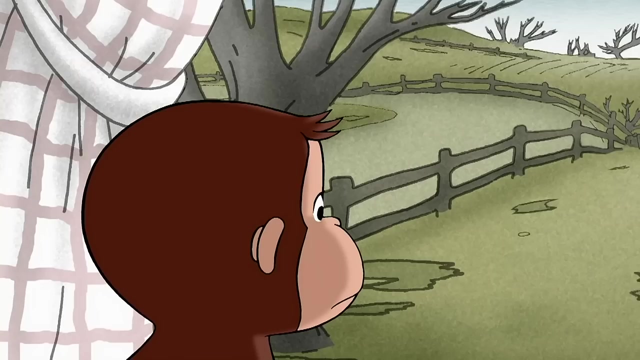 See The break's all healed. Ooh, George brought his friends back so he and Hunley could be together. George was back to normal, all right. When winter began, everything outdoors looked different. The days were short, the grass was brown and the trees were bare. 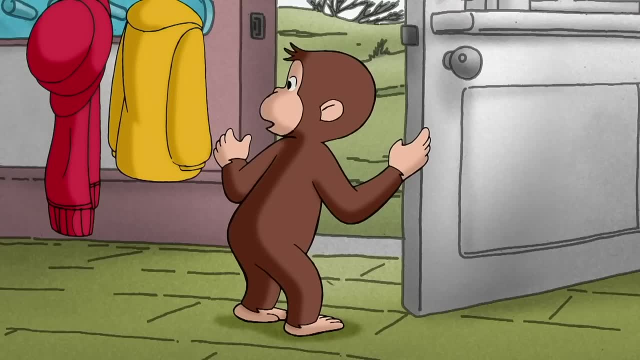 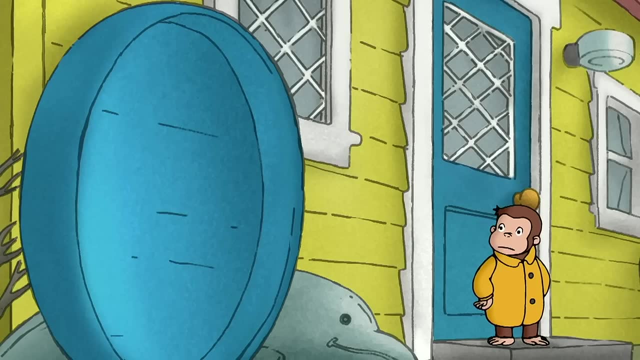 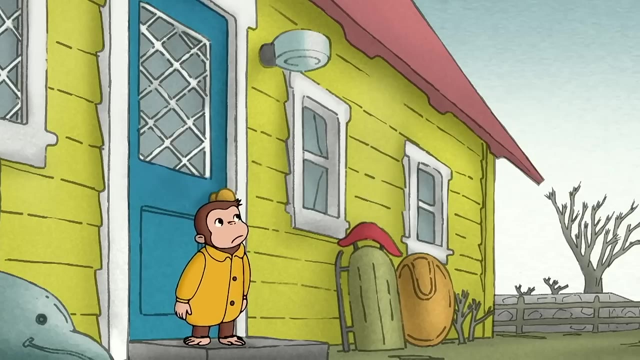 George, don't forget your coat. It may be sunny, but it's turning really cold out there. Shh George had toys for summer And toys for snow, But there were no toys for just plain cold. There weren't even birds to watch. 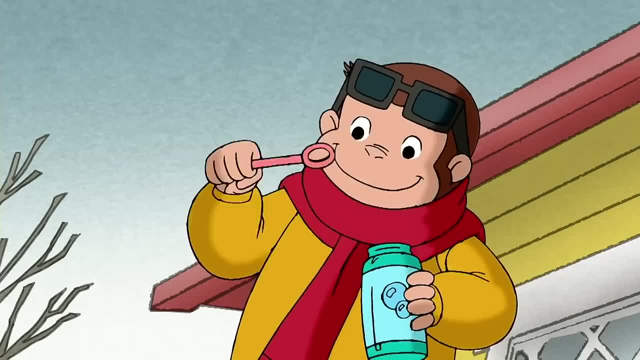 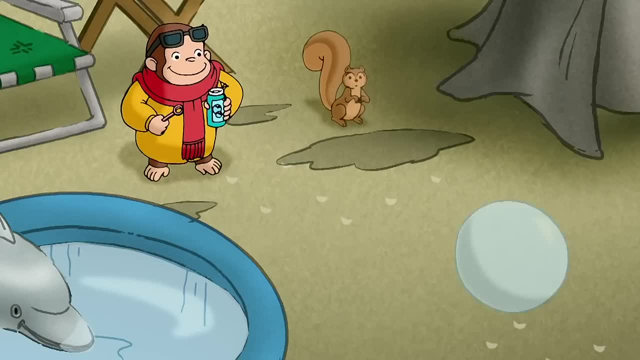 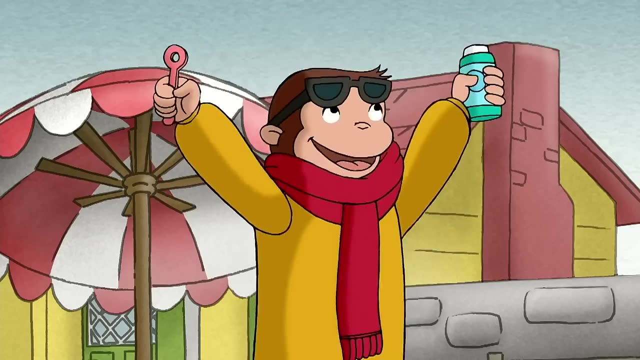 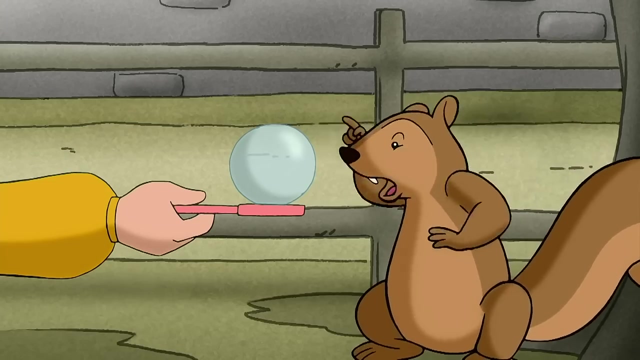 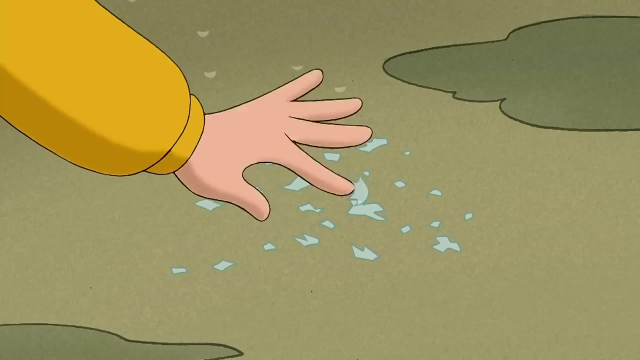 Huh, Huh, Oh, ho ho ho. Hello, George had won, He was having fun like winter had never come. Ho ho, ho, Ha ha, The bubble froze. That was pretty interesting, But it wasn't what George wanted it to do. 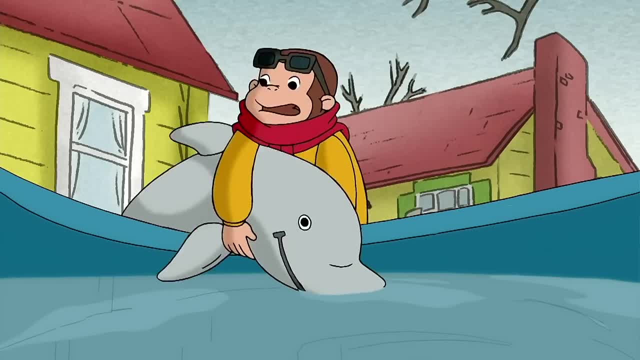 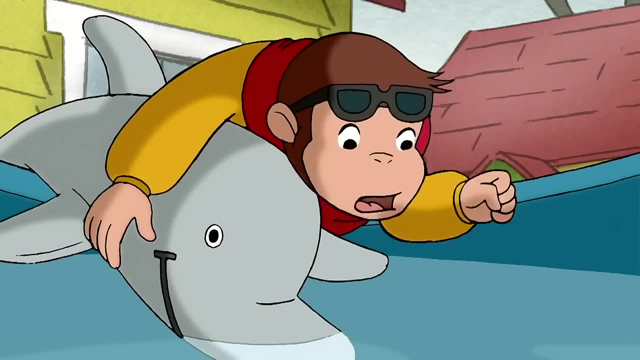 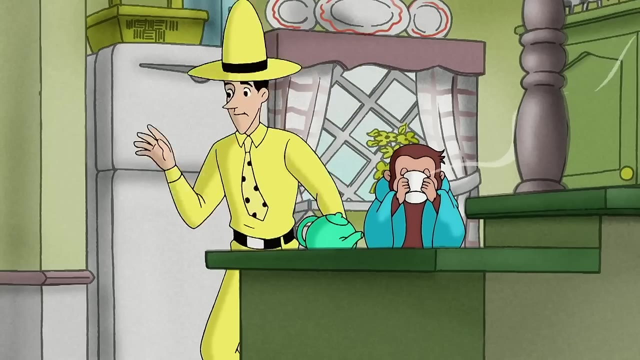 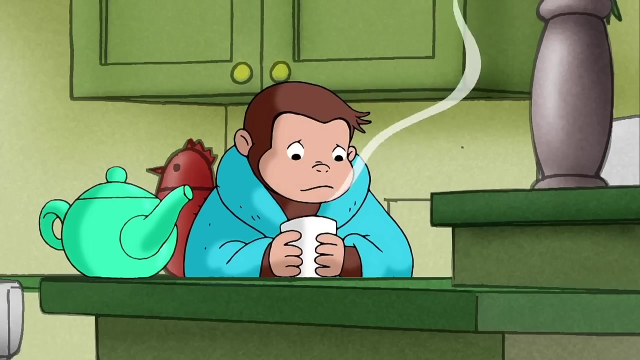 He knew his dolphin couldn't freeze. He could play with that any way he wanted. There, That'll warm you up. George was thinking two things: Hello Boy, was this Coco good? And that he was giving up. How can a monkey have any fun when his stuff all freezes up? 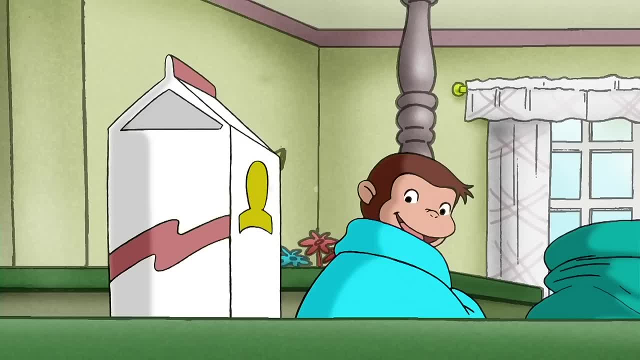 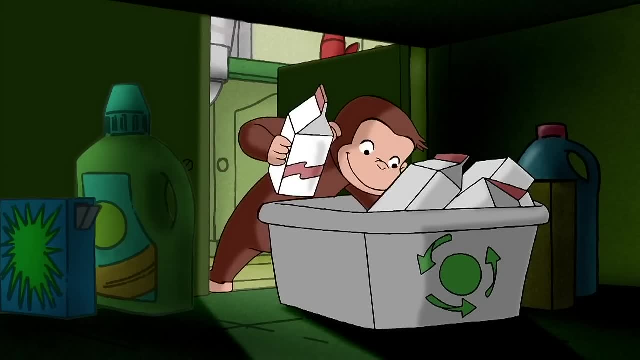 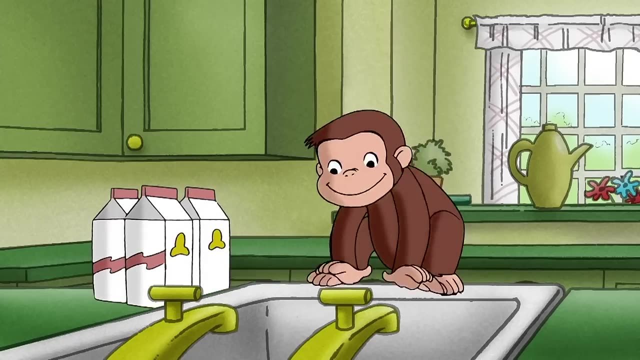 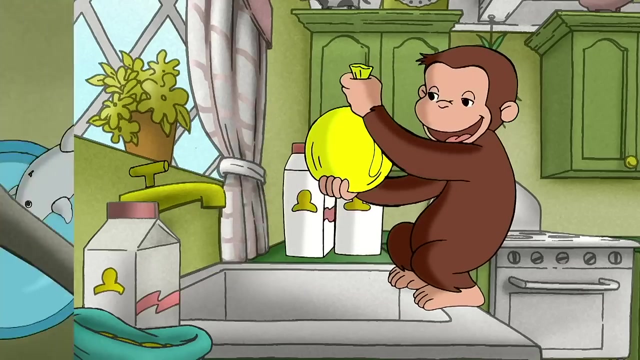 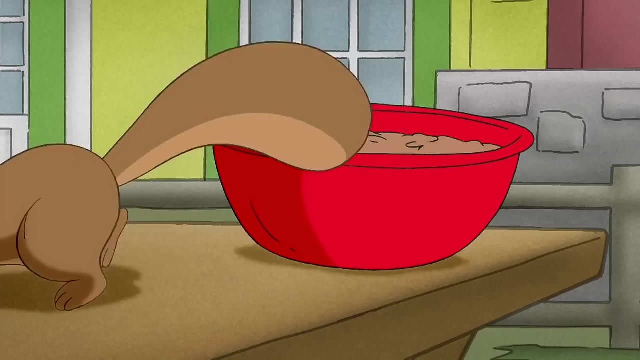 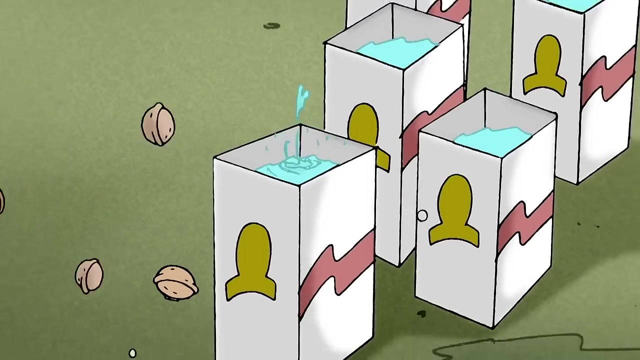 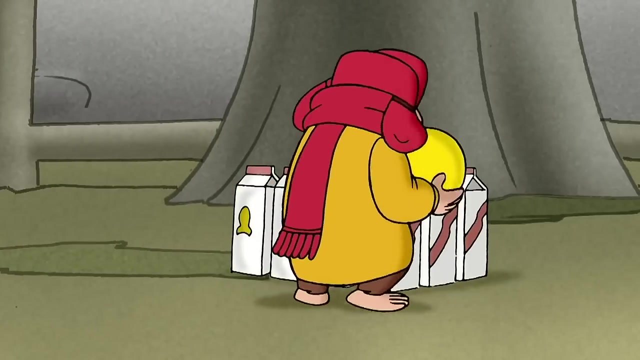 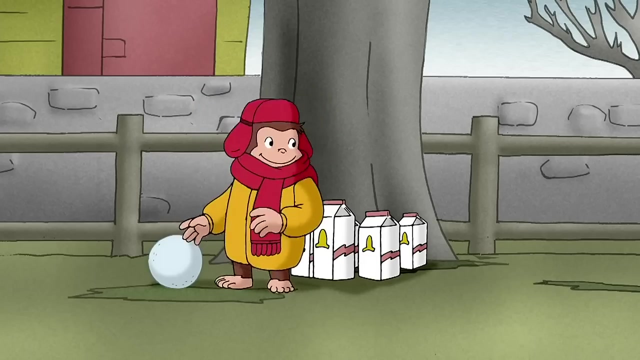